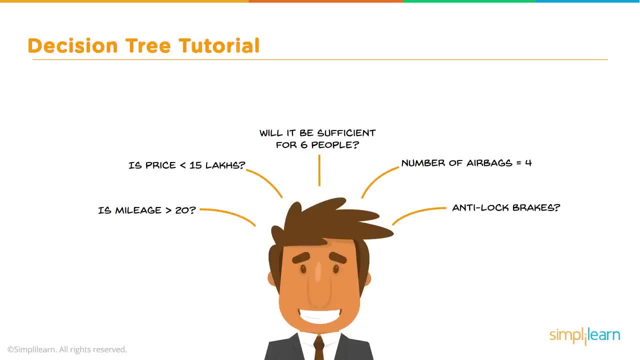 All these questions come up. Then, as we feed all this data in, we make a decision. And that decision comes up: oh hey, this seems like a good idea, Here's a car. So, as we're going through this decision process using a Decision Tree, we're going to explore this, maybe not in buying a car, but in how to process data. 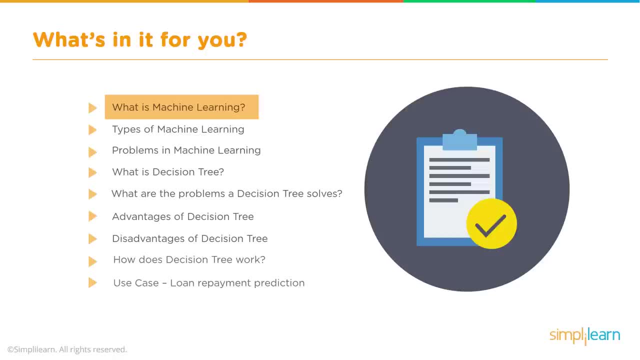 What's in it for you? Let's start by finding out what is machine learning and why we even want to know about it for processing our data, And we'll go into the three basic types of machine learning and the problems that are used by machine learning to solve. 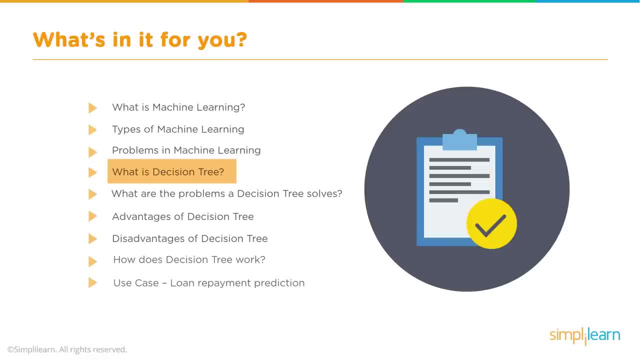 Finally, we'll get into what is a Decision Tree, What are the problems a Decision Tree solves, What are the advantages and disadvantages of using a Decision Tree? And then we want to dig in a little deep into the mechanics. How does the Decision Tree work? 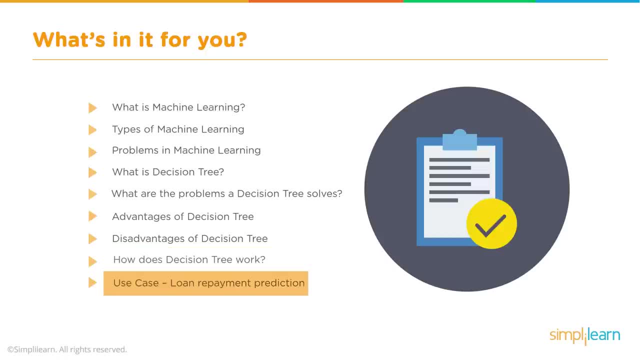 And then we'll go in and do a case loan repayment prediction, where we actually are going to put together some Python code and show you the basic Python code for generating a Decision Tree. What is machine learning? There are so many different ways to describe what is machine learning in today's world and illustrate it. 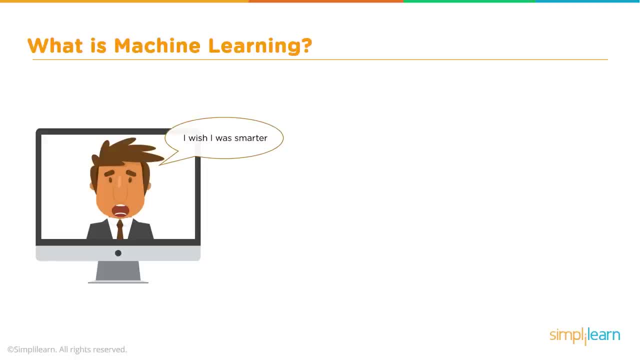 We're going to take a graphic here and making decisions or trying to understand what's going on. And really underlying machine learning is people want to wish they were smarter, wish we could understand the world better. So you can see a guy here who's saying, hey, how can I understand the world better? 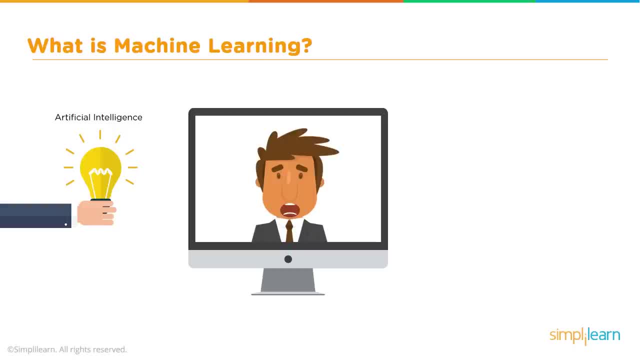 And someone comes up and says: let's use artificial intelligence. Machine learning is a part of artificial intelligence. And now he gets a big smile on his face because now he has artificial intelligence to help him, To help him make his decisions, and they can think in new ways. 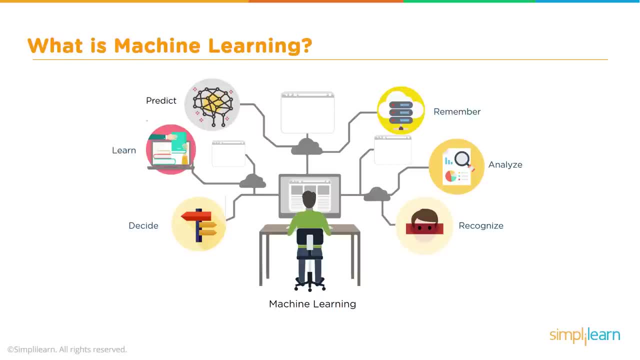 So this brings in new ideas. So what is machine learning? This is a wonderful graph. here You can see where we have a learn, predict, decide. These are the most basic three premises of machine learning. In learning, we can describe the data in new ways and be able to learn new aspects about what we're looking at. 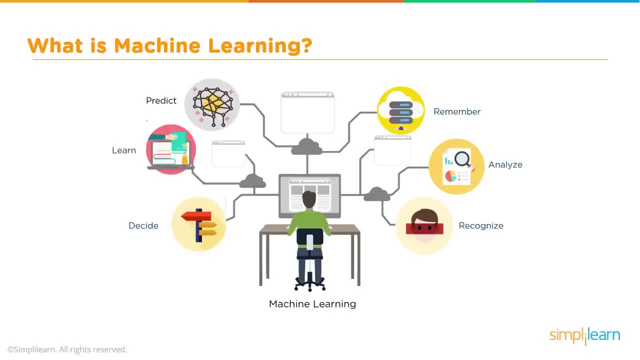 And then we can use that to predict things and we can use that to make decisions. So maybe it's something that's never happened before, but we can make a good guess whether it's going to be a good investment or not. It also helps us categorize stuff so we can remember it better. 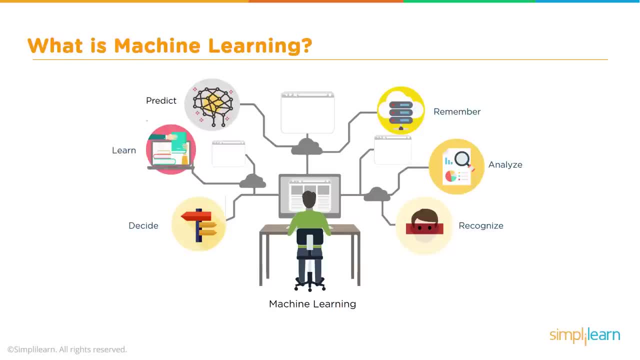 So it's easier to pull it out of the catalog. We can analyze data in new ways we never thought possible. And then, of course, there's the very large, growing industry of recognize. We can do facial recognition, driver recognition, automated car recognition. 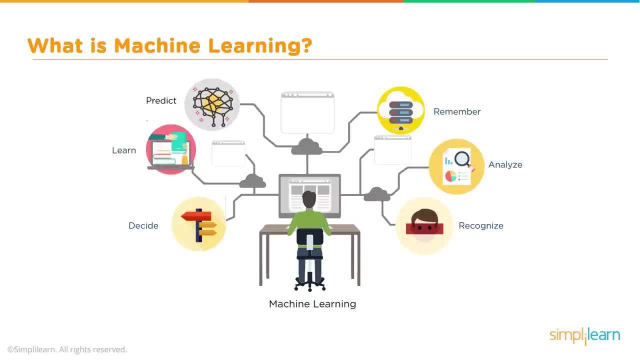 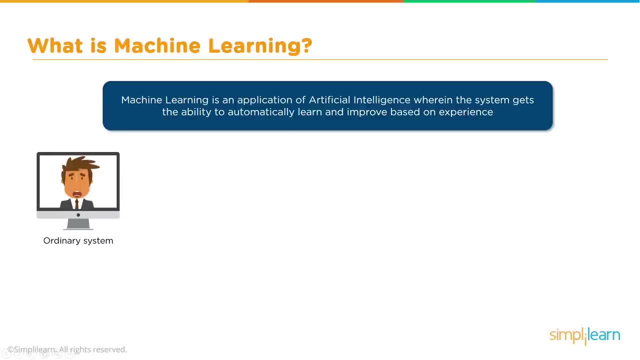 All of these are part of machine learning. Going back to our guy here who's in his ordinary system and would like to be smarter, make better choices, What happens with machine learning is an application of artificial intelligence Wherein the system gets the ability to automatically learn and improve based on experience. 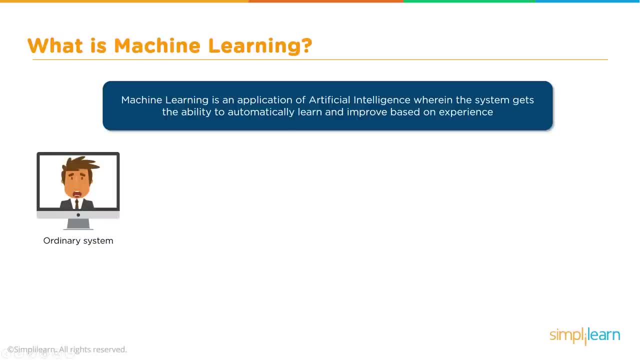 So this is exciting because you have your ordinary guy who now has another form of information coming in, And this is with the artificial intelligence. helps him see things he never saw or track things he can't track. So instead of having to read all the news feeds, he can now have an artificial intelligence sorted out. 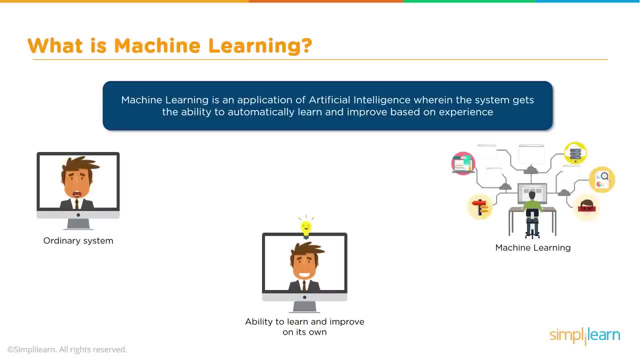 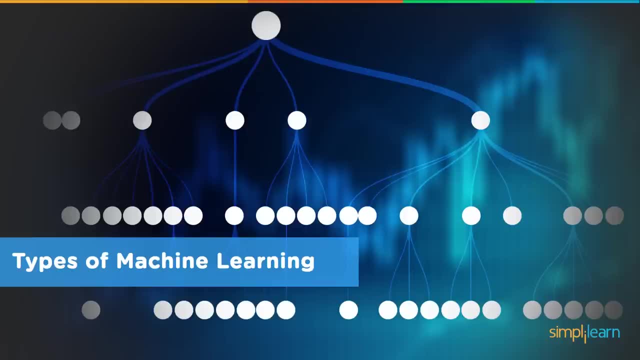 So he's only looking at the information he needs to make a choice with, And, of course, we use all those machine learning tools back in there And he's now making smarter choices with less work. Types of machine learning. Let's break it into three primary types of learning. 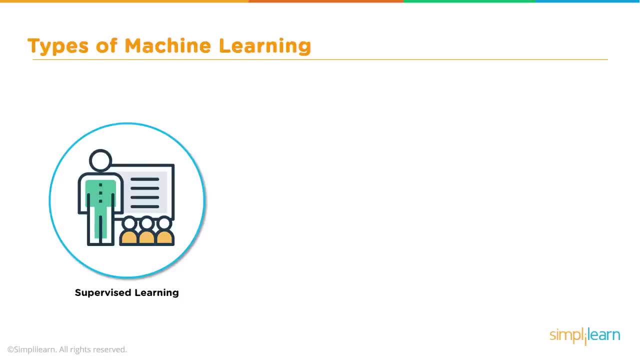 First is supervised learning, where you already have the data and the answers. So if you worked at a bank, you'd already have a list of all the previous loans and who defaulted on them and who made good payments on them. You then program your machine learning tool. 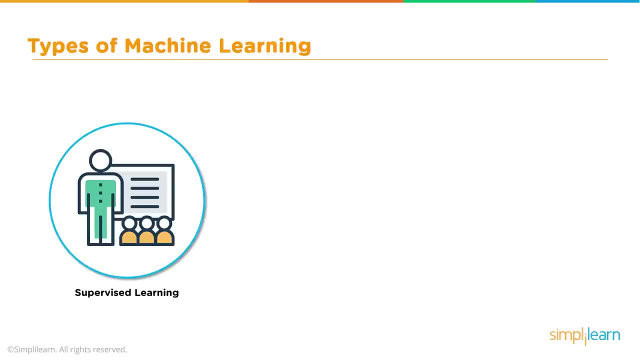 And that lets you predict on the next person whether they're going to be able to make their payments or not on their loan. If you have one category where you already know the answers, the next one would be: you don't know the answers, You just have a lot of information coming in. 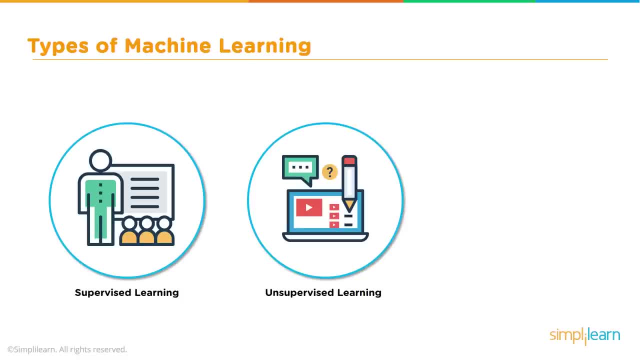 Unsupervised learning allows you to group liked information together. So if you're analyzing photos, it might group all the images of trees together and all the images of houses together, without ever knowing what a house or a tree is. Which leads us to the third type of machine learning. 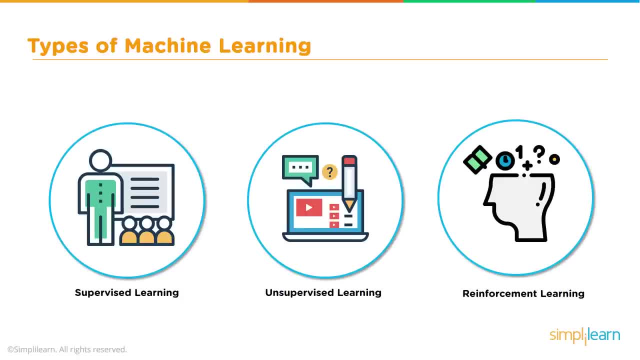 The third type of machine learning is reinforcement learning. Unlike supervised or unsupervised learning, you don't have the data Prior to starting, So you get the data one line at a time And then, whether you make a good choice or a bad choice, the machine learning tool has to then adjust accordingly. 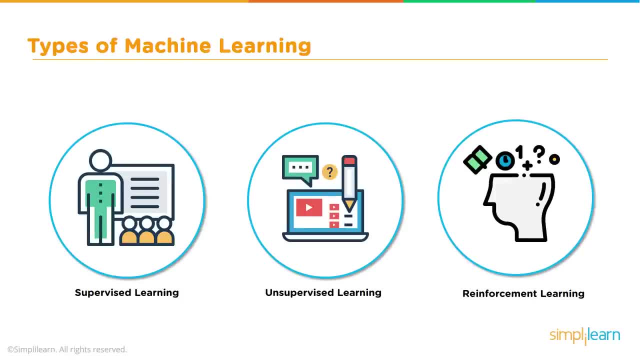 So you get a plus or minus feedback. You can liken this to the way a human learns. We experience life one minute at a time and we learn from that, And either our memory is good or we learn to avoid something. Problems in machine learning. 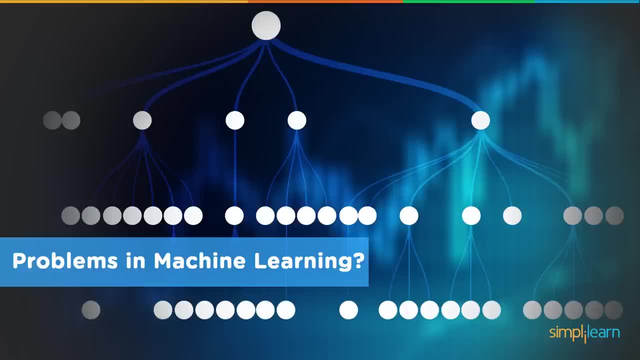 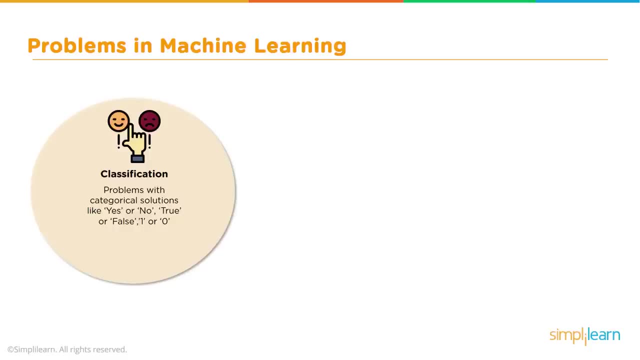 To understand where the decision tree fits into our machine learning tools, we have to understand the basics of some of the machine learning problems, And three of the primary ones fall underneath classification Problems with categorical solutions like yes or no, true or false, one or zero. 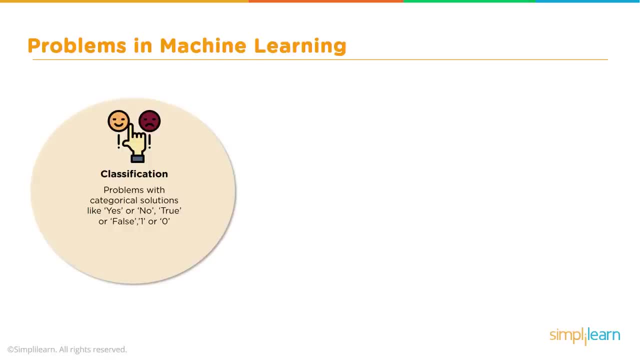 This might be: does it belong to a particular group, yes or no? Then we have regression Problems, where there's a continuous value need to be predicted, like product prices, profit, And you can see here- this is a very simple linear graph. 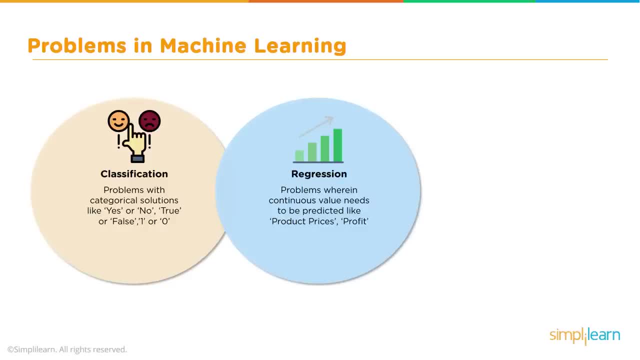 You can guess what the next value is based on the first four. It kind of follows a straight line going up And clustering. This is problems where the data needs to be organized to find specific patterns, Like in the case of product recommendation. They group all the different products that people just like you viewed on a shopping site. 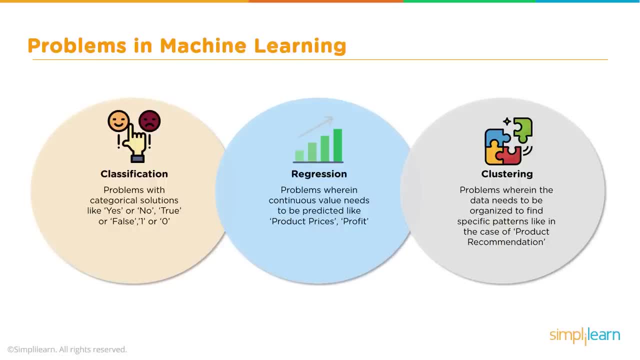 And say: people who bought this also bought this. The most commonly used for the decision tree is for classification, For figuring out is it red or is it not, Is it a fruit or is it a vegetable, Yes or no, True or false. 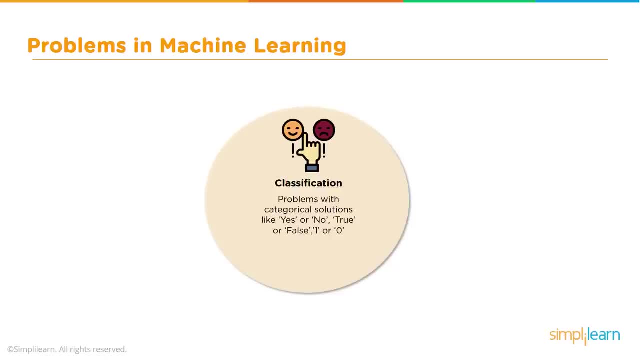 Left or right, Zero or one, And so when we talk about classification, we're going to look at the basic machine learning. These are the four main tools used in classification: There's NAVE, Bayes, logistic regression, decision tree and random forest. 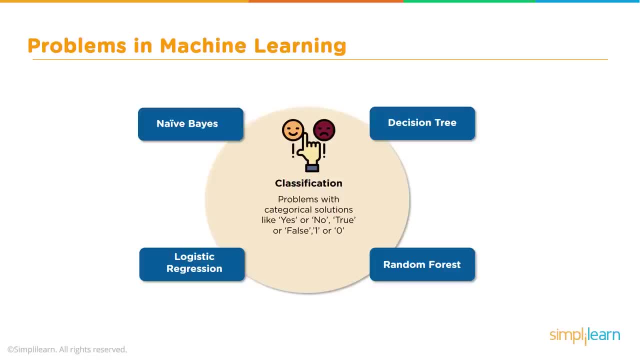 The first two are for simpler data, So if your data is not very complex, you can usually use these to do a fairly good representation by drawing a line through the data or a curve through the data. They work wonderful in a lot of problems. 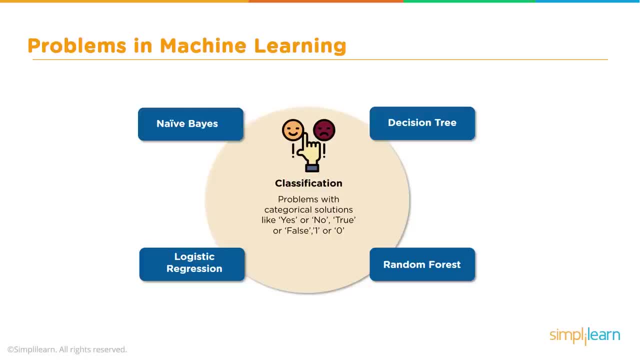 But as things get more complicated, the decision tree comes in, And then, if you have a very large amount of data, You start getting into the random forest. So the decision tree is actually a part of the random forest, But today we're just going to focus on the decision tree. 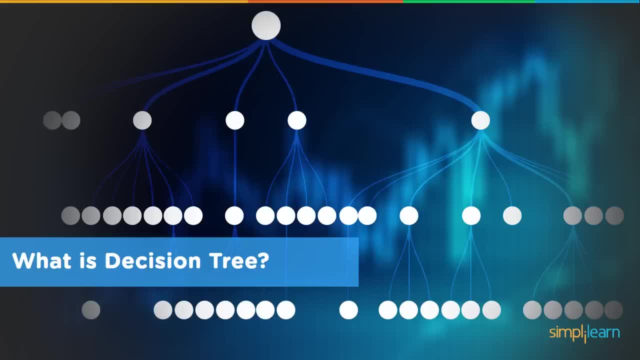 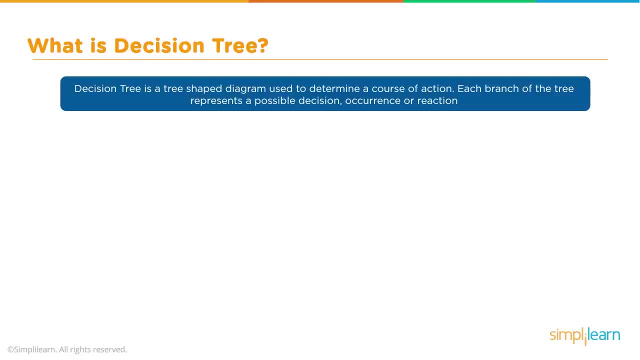 What is a decision tree? Let's go through a very simple example before we dig in deep. Decision tree is a tree-shaped diagram used to determine a course of action. Each branch of the tree represents a possible decision, occurrence or reaction. Let's start with a simple question. 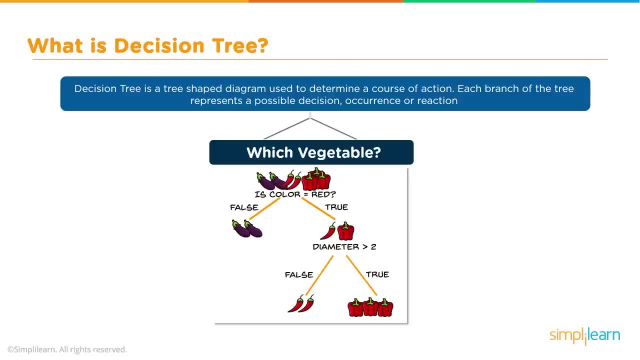 How to identify a random vegetable from a shopping bag. So we have this group of vegetables in here And we can start off by asking a simple question: is it red? And if it's not, then it's going to be the purple fruit to the left, probably an eggplant. 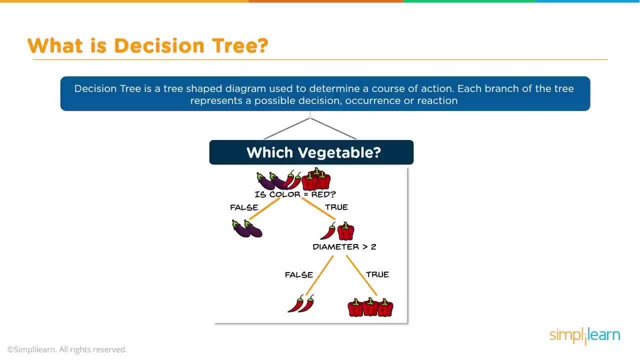 If it's true, it's going to be one of the red fruits. Is the diameter greater than two? If false, it's going to be what looks to be a red chili, And if it's true, it's going to be a bell pepper from the capsicum family. 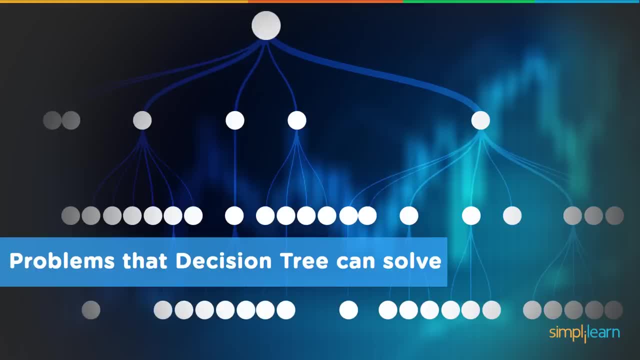 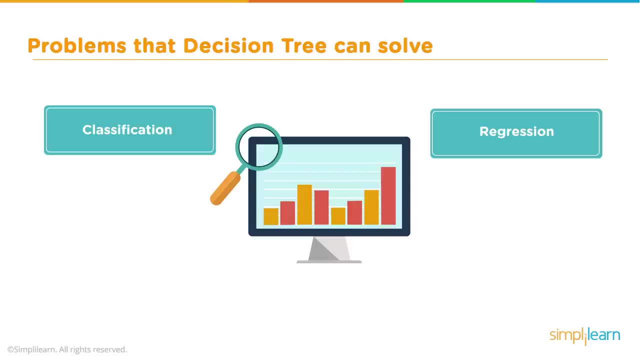 So it's a capsicum Problems that decision tree can solve. So let's look at the two different categories the decision tree can be used on. It can be used on the classification- The true, false, yes, no- And it can be used on regression, where we figure out what the next value is in a series of numbers or a group of data. 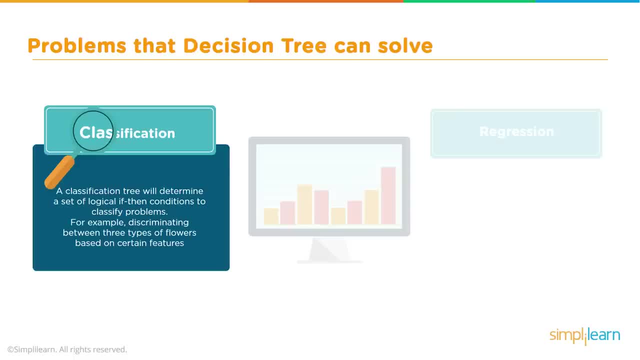 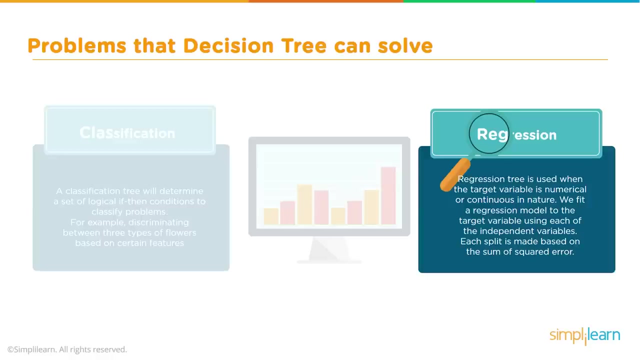 In classification: the classification tree will determine a set of logical, if then conditions to classify problems, For example discriminating between three types of flowers based on certain features. In regression: a regression tree is used when the target variable is numerical or continuous in nature. 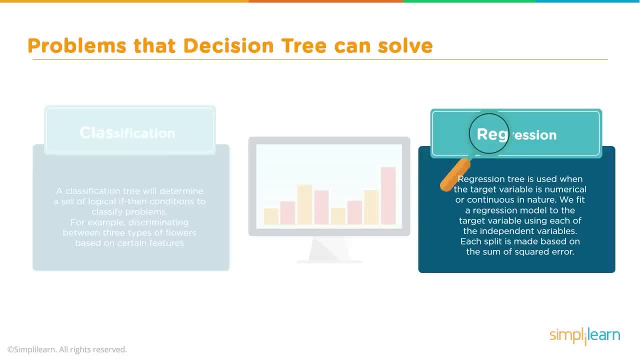 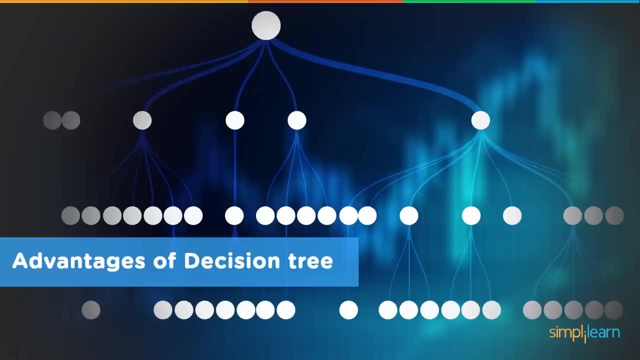 We fit the regression model to the target variable using each of the independent variables. Each split is made based on the sum of squared error. Before we dig deeper into the mechanics of the decision tree, let's take a look at the advantages of using a decision tree. 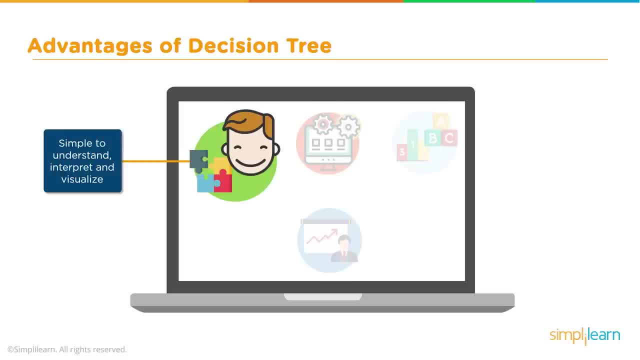 And we'll also take a glimpse at the disadvantages. The first thing you'll notice is that it's simple to understand, interpret and visualize. It really shines here because you can see exactly what's going on in a decision tree. Little effort is required for data preparation. 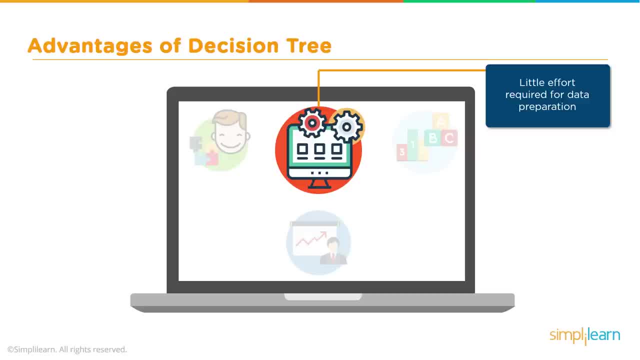 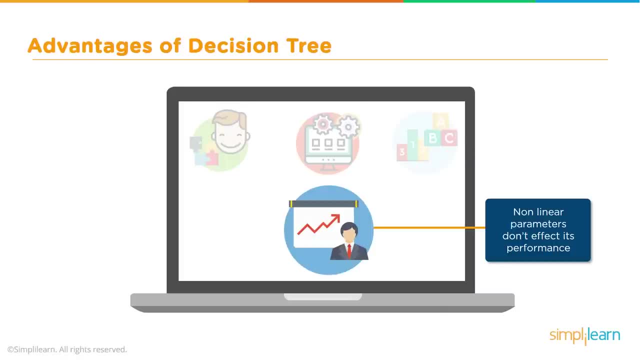 So you don't have to do special scaling. There's a lot of things you don't have to worry about when using a decision tree. It can handle both numerical and categorical data, as we discovered earlier, And nonlinear parameters don't affect its performance. 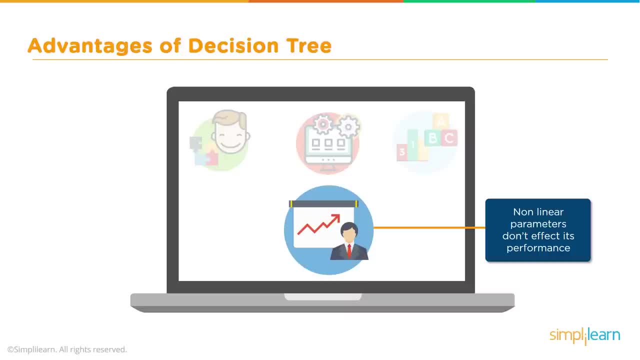 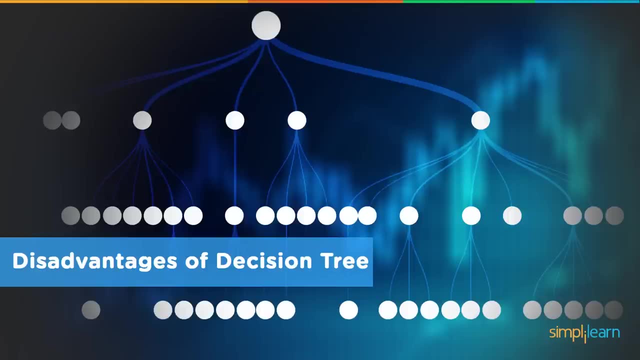 So even if the data doesn't fit an easy curved graph, you can still use it to create an effective decision or prediction. If we're going to look at the advantages of a decision tree, we also need to understand the disadvantages of a decision tree. 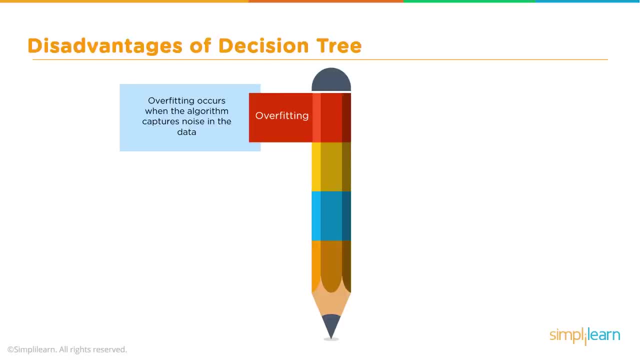 The first disadvantage is overfitting. Overfitting occurs when the algorithm captures noise in the data. That means you're solving for one specific instance instead of a general solution for all the data. High variance: The model can get unstable due to small variation in data. 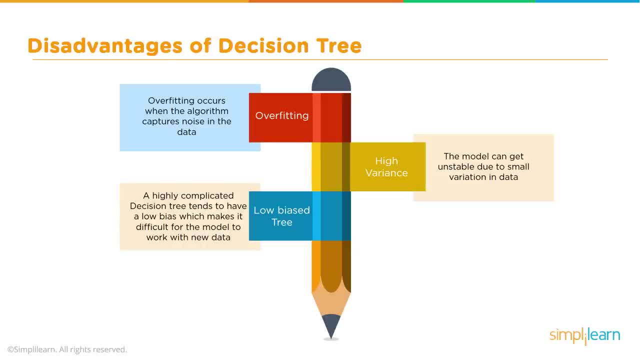 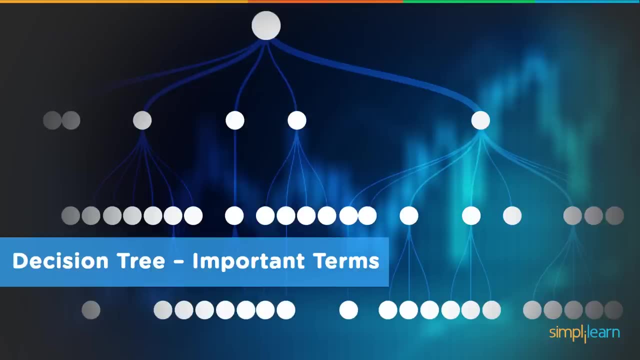 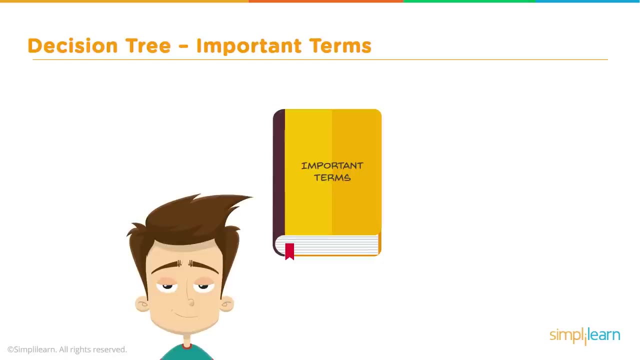 Low bias tree. A highly complicated decision tree tends to have a low bias, which makes it difficult for the model to work with new data. Decision tree important terms. Before we dive in further, we need to look at some basic terms. We need to have some definitions to go with our decision tree. 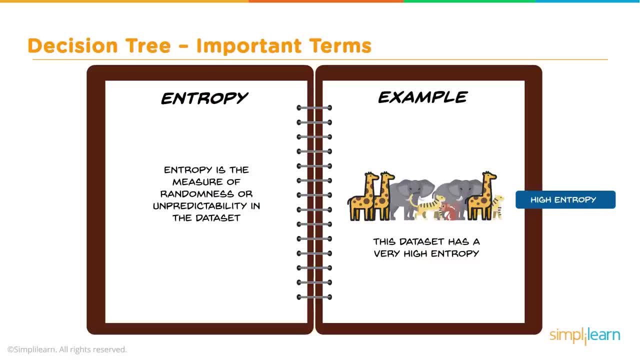 and the different parts we're going to be using. We'll start with entropy. Entropy is a measure of randomness or unpredictability in the data set. For example, we have a group of animals In this picture. there's four different kinds of animals. 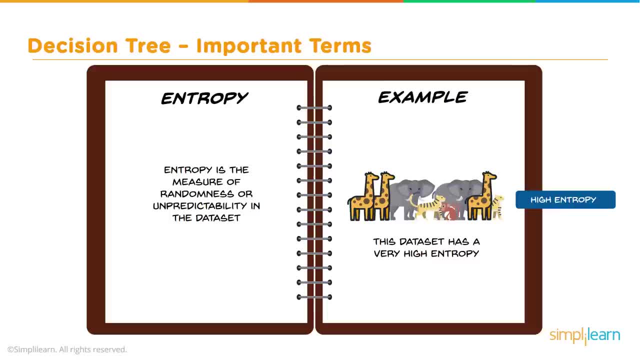 And this data set is considered to have a high entropy. You really can't pick out what kind of animal it is based on looking at just the four animals as a big clump of entities. So as we start to look at this, we start splitting it into subgroups. 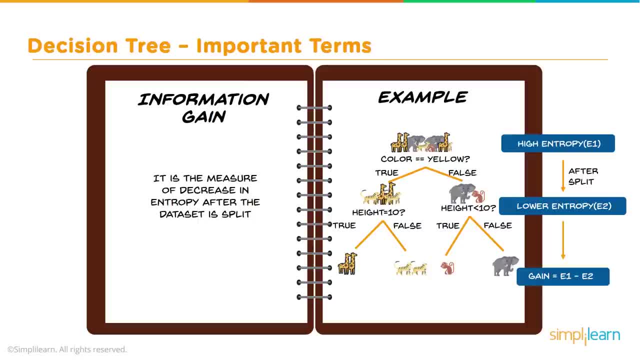 We come up with our second definition, which is information gain. Information gain: It is a measure of decrease in entropy after the data set is split. So in this case, based on the color yellow, we've split one group of animals on one side, as true. 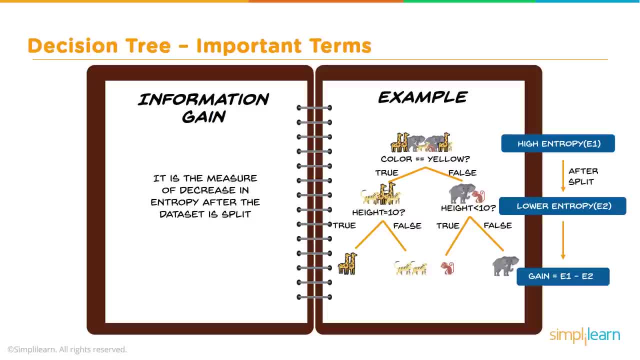 and those who aren't yellow as false. As we continue down the yellow side, we split based on the height. True or false equals 10. And on the other side, height is less than 10.. True or false. And, as you see, as we split it, 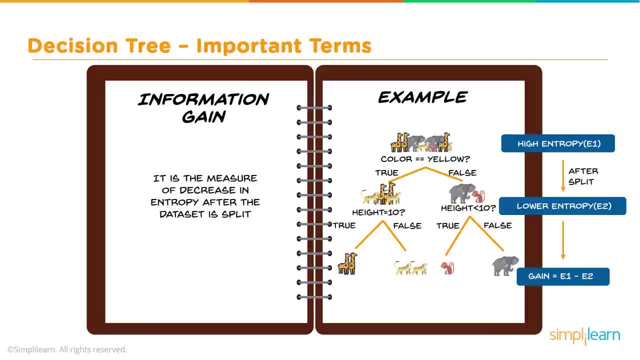 the entropy continues to be less and less and less, And so our information gain is simply the entropy, E1 from the top and how it's changed to E2 in the bottom, And we'll look at the deeper math, although you really don't need to know a huge amount of math. 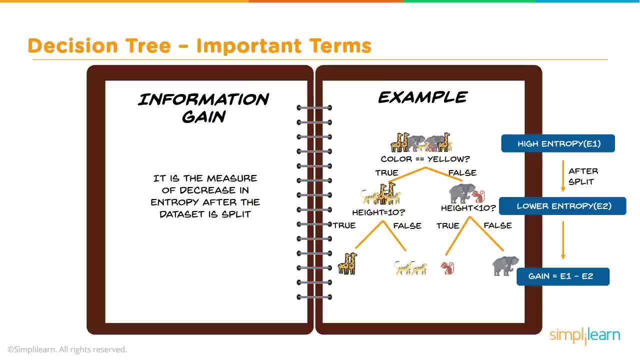 when you actually do the programming in Python, because they'll do it for you, But we'll look on the actual math, at how they compute entropy. Finally, we want to know the different parts of our tree And they call the leaf node. Leaf node carries the classification or the decision. 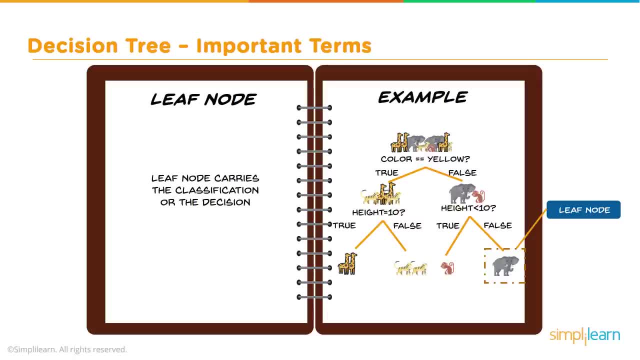 So it's the final end. at the bottom Decision node has two or more branches. This is where we're breaking the group up into different parts And finally you have the root node. The topmost decision node is known as the root node. 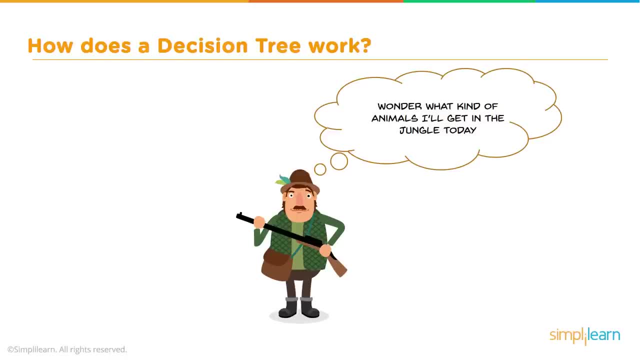 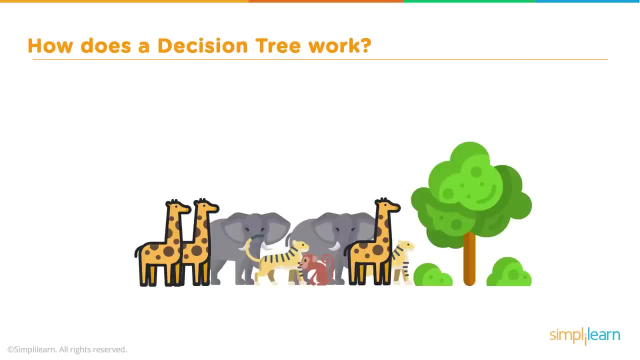 How does a decision tree work? Wonder what kind of animals I'll get in the jungle today. Maybe you're the hunter with the gun, or, if you're more into photography, you're a photographer with a camera. So let's look at this group of animals. 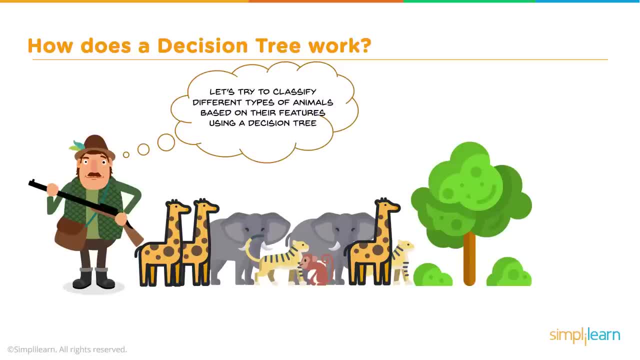 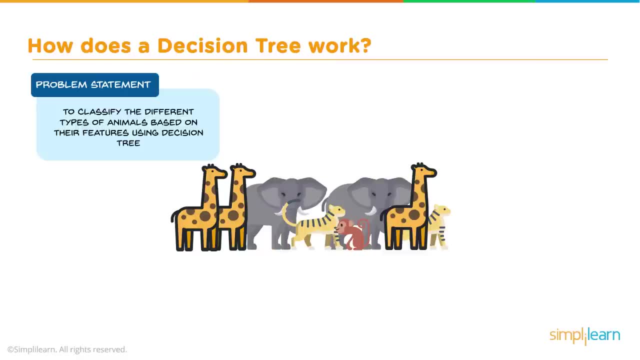 and let's try to classify different types of animals based on their features using a decision tree. So the problem statement is to classify the different types of animals based on their features using a decision tree. The data set is looking quite messy and the entropy is high in this case. 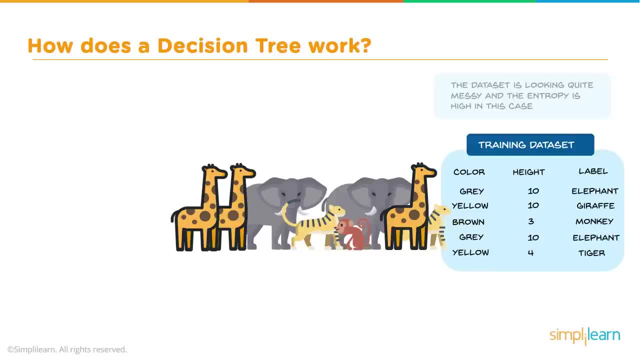 So let's look at a training set or a training data set, And we're looking at color, We're looking at height, And then we have our different animals. We have our elephants, our giraffes, our monkeys and our tigers. 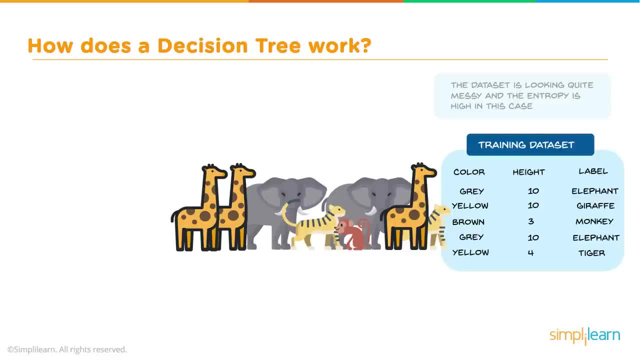 And they're of different colors and shapes. Let's see what that looks like. And how do we split the data. We have to frame the conditions that split the data in such a way that the information gain is the highest. Note gain is the measure of decrease in entropy after splitting. 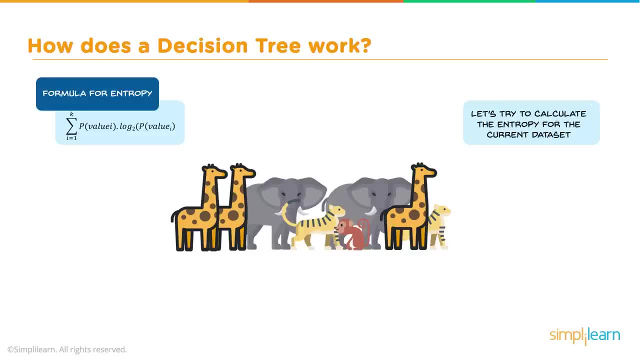 So the formula for entropy is the sum. that's what this symbol looks like. it looks kind of like a funky E of k where i equals 1 to k. k would represent the number of animals, the different animals in there, where value or p value of i. 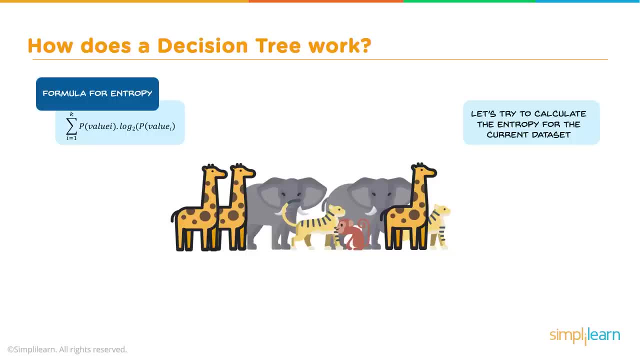 would be the percentage of that animal times the log base 2 of the same the percentage of that animal. Let's try to calculate the entropy for the current data set and take a look at what that looks like, And don't be afraid of the math. 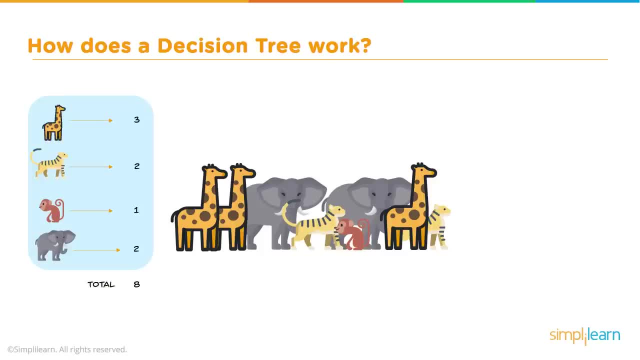 You don't really have to memorize this math, Just be aware that it's there and this is what's going on in the background. And so we have 3 giraffes, 2 tigers, 1 monkey, 2 elephants. 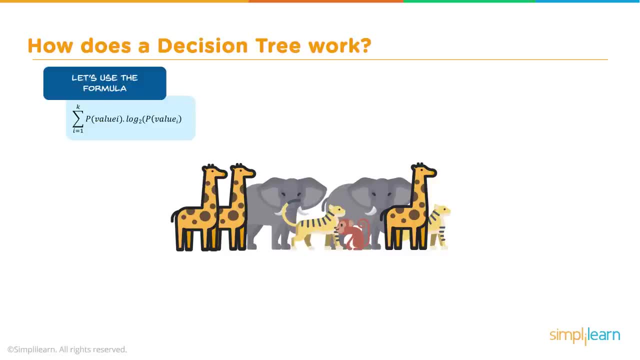 A total of 8 animals gathered And if we plug that into the formula we get an entropy that equals 3 over 8.. So we have 3 giraffes, a total of 8, times the log. Usually they use base 2 on the log. 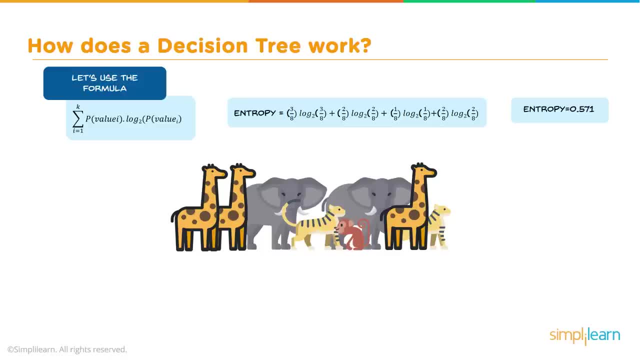 So log base 2 of 3 over 8 plus, in this case let's say it's the elephants 2 over 8, 2 elephants over a total of 8, times log base 2, 2 over 8,. 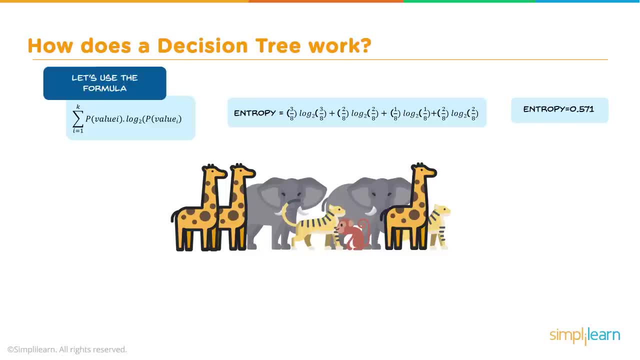 plus 1 monkey over a total of 8, log base 2, 1 over 8, and plus 2 over 8 of the tigers, log base 2 over 8.. And if we plug that into our computer or calculator, 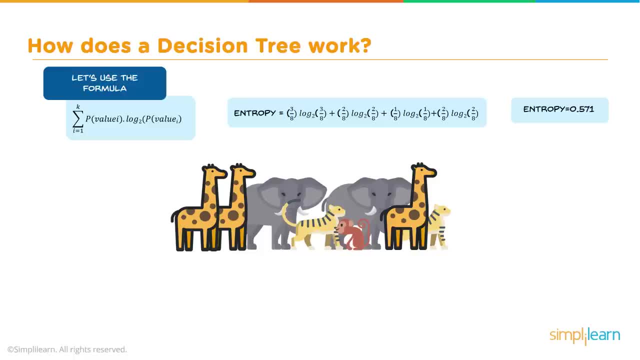 I obviously can't do logs. in my head we get an entropy equal to 0.571.. The program will actually calculate the entropy of the data set similarly after every split to calculate the gain. Now we're not going to go through each set, one at a time. 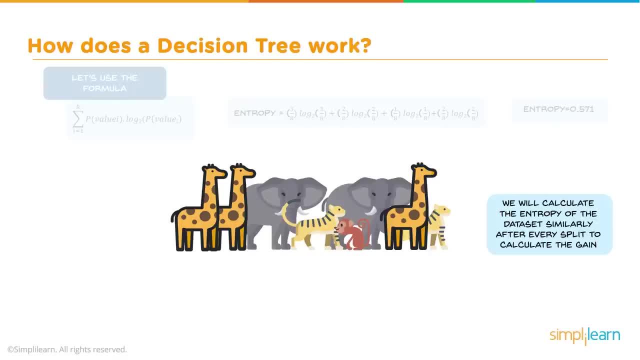 to see what those numbers are. We just want you to be aware that this is a formula or the mathematics behind it. Gain can be calculated by finding the difference of the subsequent entropy values after a split. Now we will try to choose a condition that gives us the highest gain. 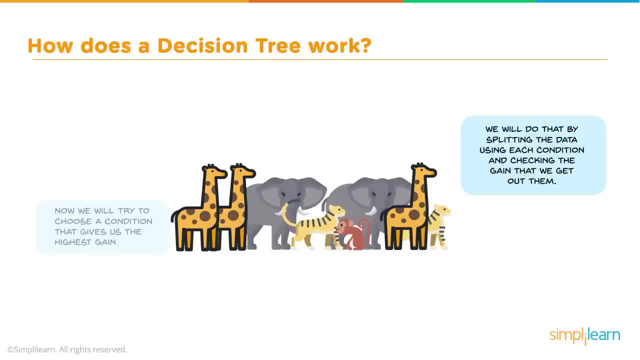 We will do that by splitting the data using each condition and checking that the gain we get out of them The condition that gives us the highest gain to make the first split. Can you guess what that first split will be just by looking at this image. 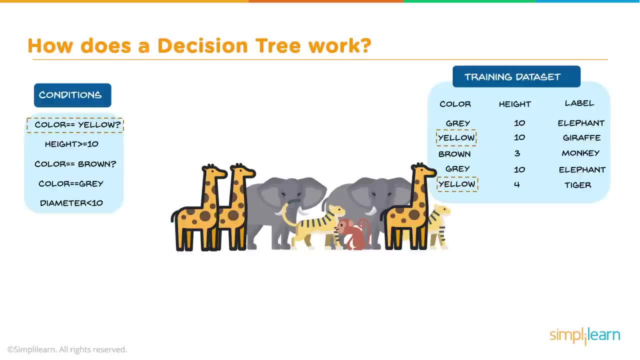 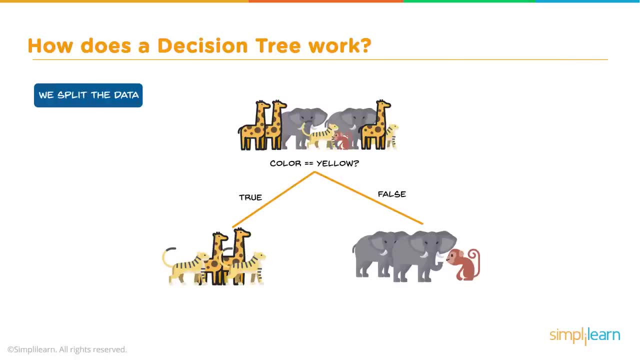 As a human, it's probably pretty easy to split it. Let's see if you're right. If you guessed the color yellow, you're correct. Let's say the condition that gives us the maximum gain is yellow. So we will split the data based on the color yellow. 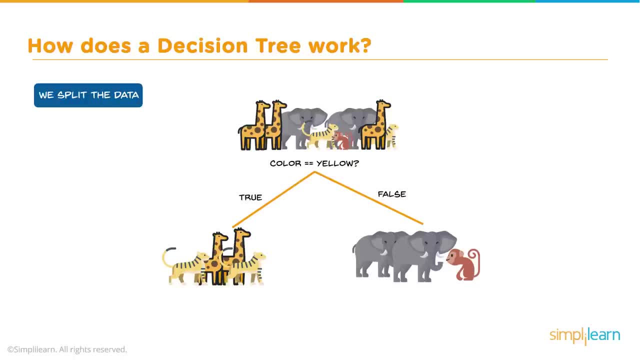 If it's true, that group of animals goes to the left. If it's false, it goes to the right. The entropy after the splitting has decreased considerably. However, we still need some splitting to have both the branches to attain an entropy value equal to zero. 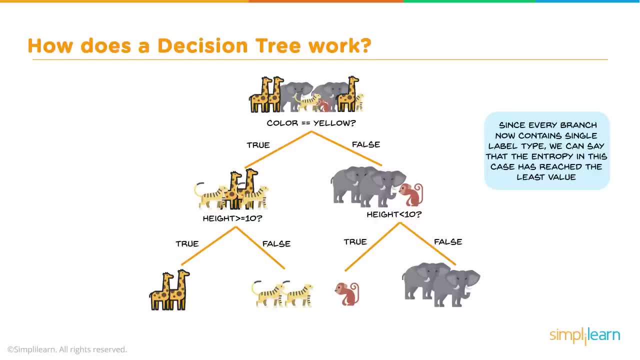 So we decide to split both the nodes, using height as the condition. Since every branch now contains single label type, we can say that entropy, in this case, has reached the least value. And here you see, we have the giraffes, the tigers, the monkey and the elephants. 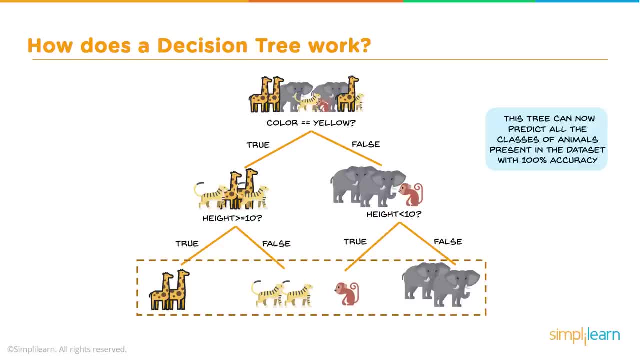 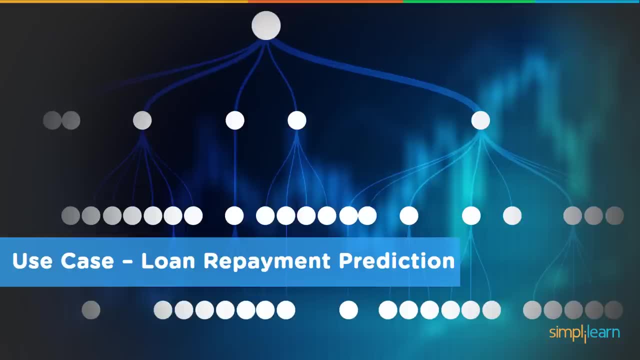 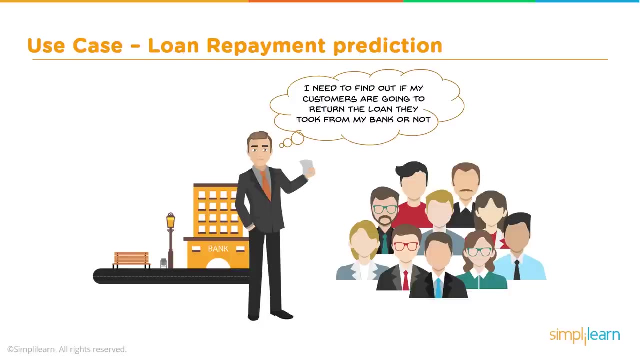 all separated into their own groups. This tree can now predict all the classes of animals present in the data set with 100% accuracy. That was easy. Use Case Loan Repayment Prediction and open up some Python and see what the programming code and the scripting looks like. 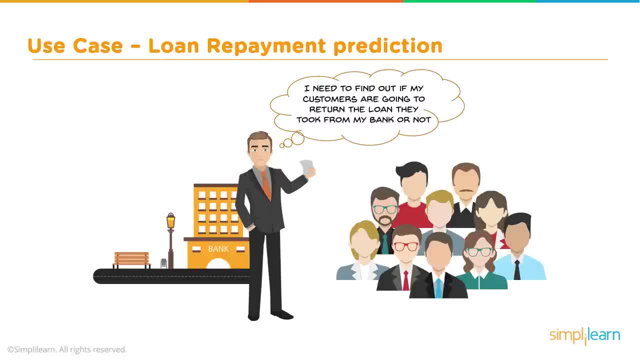 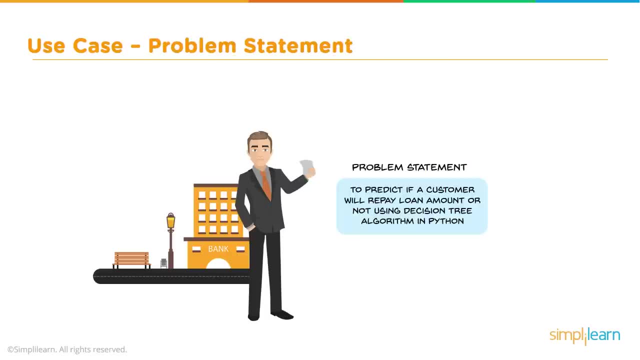 In here we're going to want to do a prediction, And we start with this individual here who's requesting to find out how good his customers are going to be, whether they're going to repay their loan or not for his bank, And from that we want to generate a problem statement. 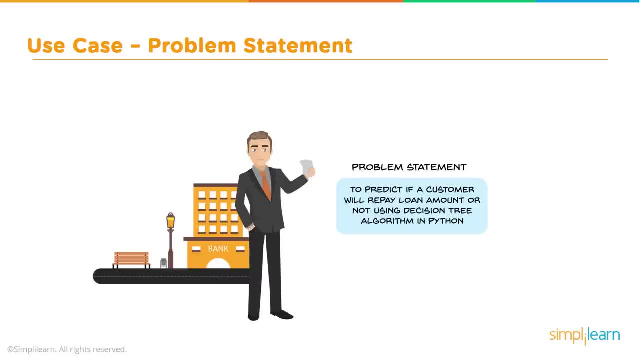 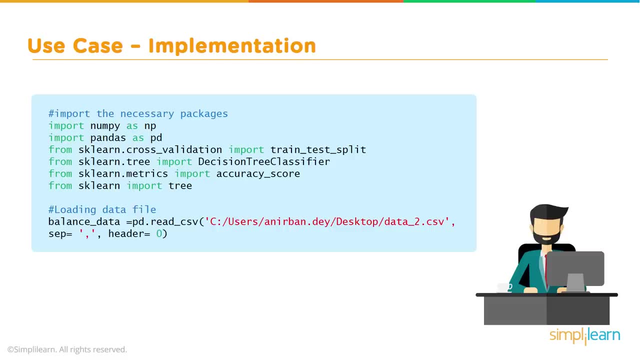 to predict if a customer will repay a loan amount or not, And then we're going to be using the decision tree algorithm in Python. Let's see what that looks like and let's dive into the code In our first few steps of implementation. 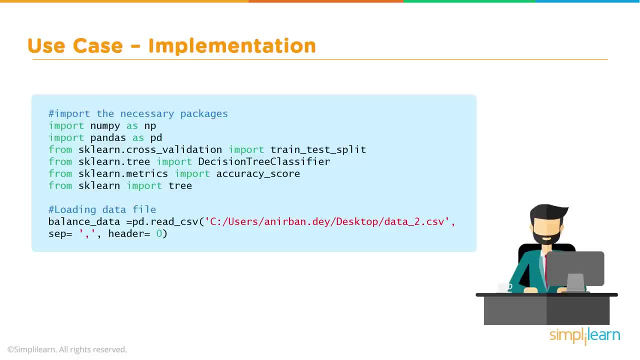 we're going to start by importing the necessary packages that we need from Python, And we're going to load up our data and take a look at what the data looks like. So the first thing I need is I need something to edit my Python and run it in. 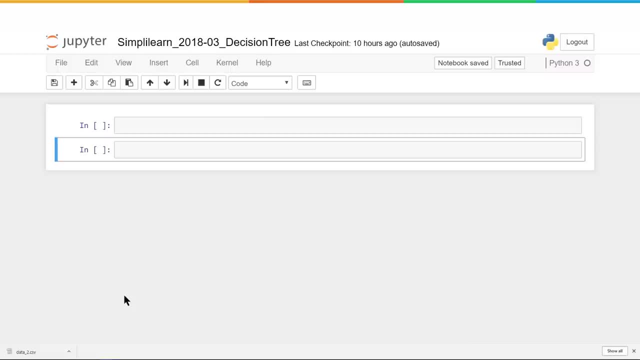 So let's flip on over, And here I'm using the Anaconda Jupyter Notebook. Now you can use any Python IDE you like to run it in, But I find the Jupyter Notebook's really nice for doing things on the fly, And let's go ahead and just paste that code in the beginning. 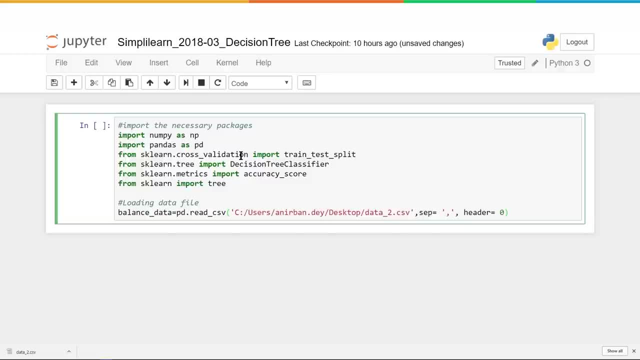 And before we start let's talk a little bit about what we're bringing in. There's a couple things in here. I have to make a couple changes as we go through this first part of the import. The first thing we bring in is numpy as np. 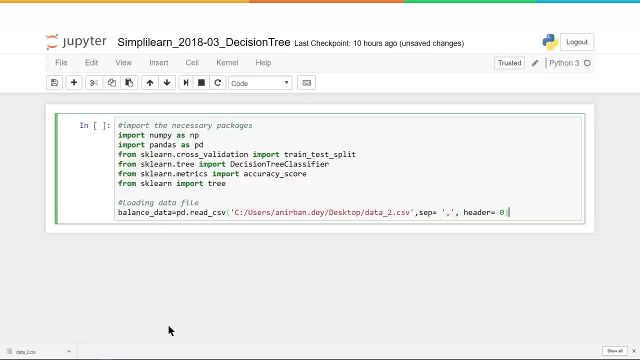 That's very standard When we're dealing with mathematics, especially with very complicated machine learning tools. you almost always see the numpy come in for your numbers. It's called number Python. It has your mathematics in there. In this case, we actually could take it out. 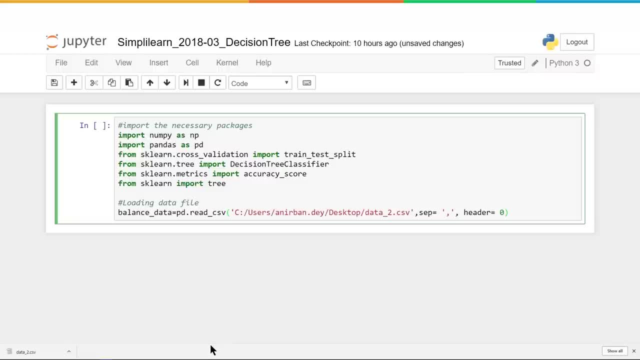 But generally you'll need it for most of your different things you work with, And then we're going to use pandas as pd. This is a data frame setup, And you can liken this to taking your basic data and storing it in a way that looks like. 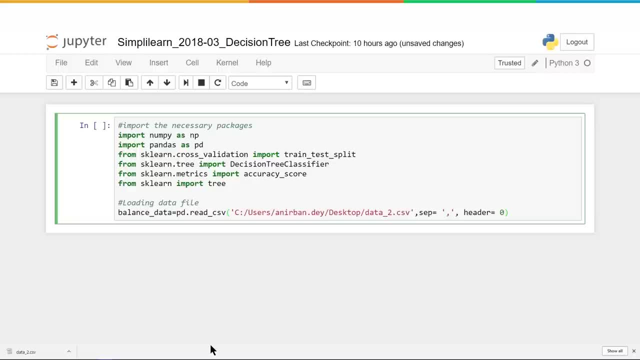 an Excel spreadsheet. So as we come back to this, when you see np or pd, those are very standard uses- you'll know that that's the pandas And I'll show you a little bit more when we explore the data in just a minute. 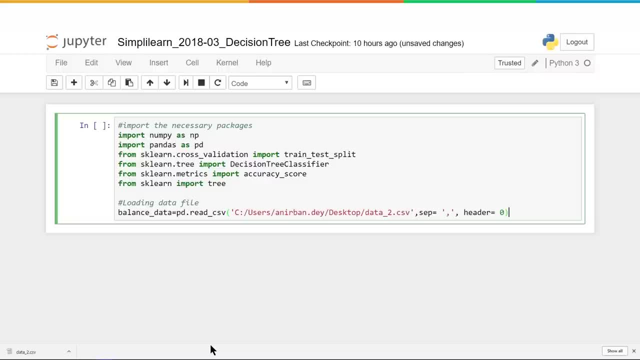 Then we're going to need to split the data. So I'm going to bring in our train, test and split And this is coming from the sklearn package: cross-validation. In just a minute we're going to change that. We're going to need the sktree import. 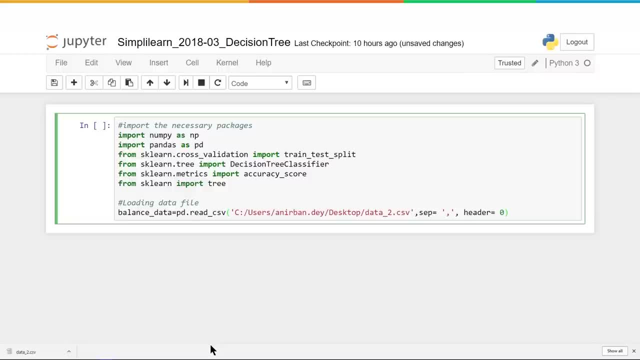 decision tree classifier. That's the actual tool we're using. Remember, I told you don't be afraid of the mathematics, It's going to be done for you. Well, the decision tree classifier has all that mathematics in there for you, So you don't have to figure it back out again. 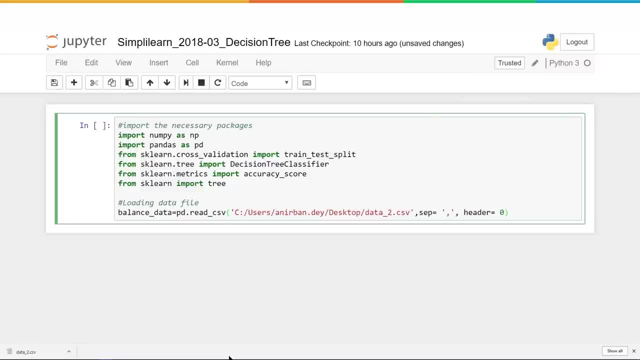 And then we have sklearnmetrics for accuracy score. We need to score our setup. That's the whole reason we're splitting it between the training and testing data. And finally, we still need the sklearn import tree, And that's just the basic tree function. 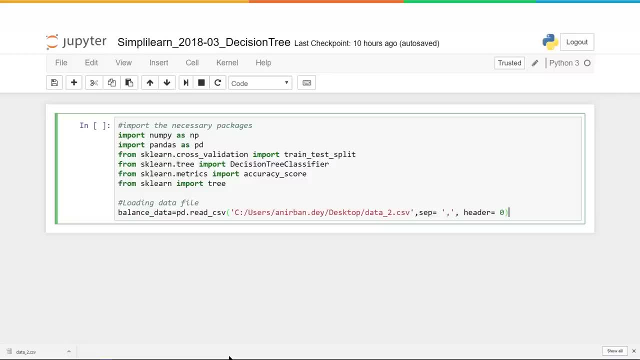 that's needed for the decision tree classifier. We're going to load our data down here And I'm going to run this And we're going to get two things on here: One, we're going to get an error And two, we're going to get a warning. 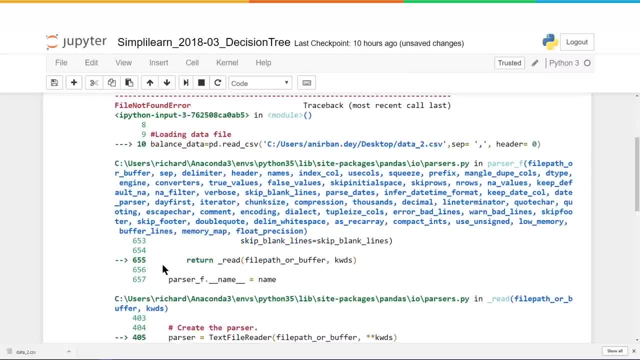 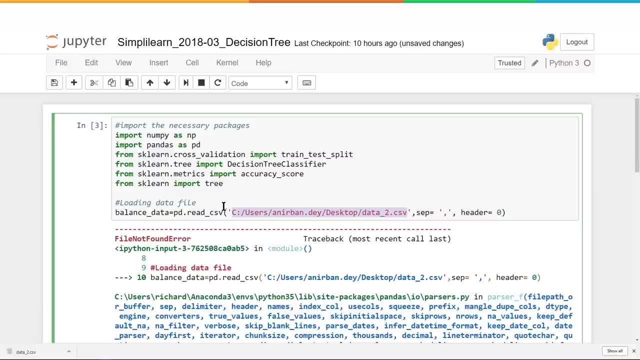 Let's see what that looks like. So the first thing we had is: we have an error. Why is this error here? Well, it's looking at this and says: I need to read a file, And when this was written, the person who wrote it. 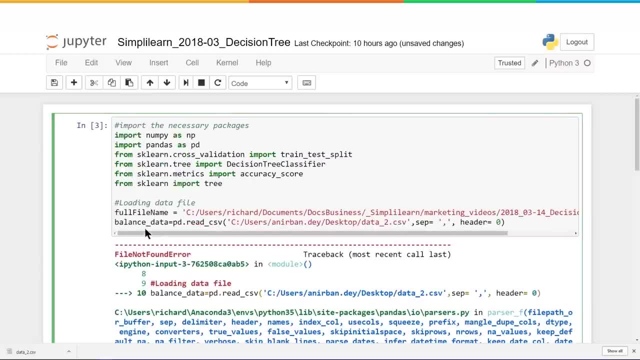 this is their path where they stored the file. So let's go ahead and fix that And I'm going to put in here a full name And you'll see. it's on my C drive and there's this very lengthy setup on here where I stored the data2.csv file. 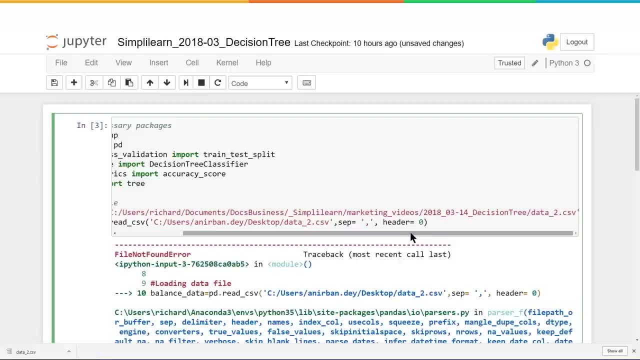 Don't worry too much about the full path, because on your computer it will be different. The data.2.csv file was generated by SimplyLearn. If you want a copy of that, you can comment down below and request it here in the YouTube. 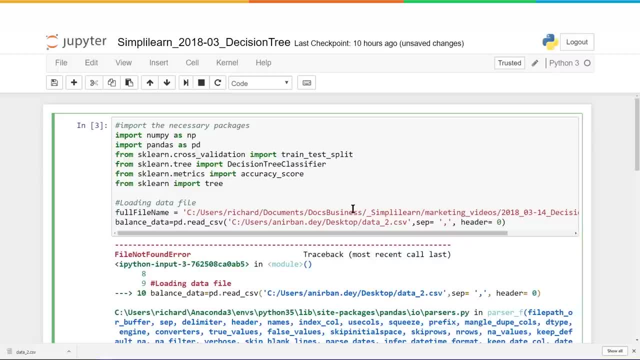 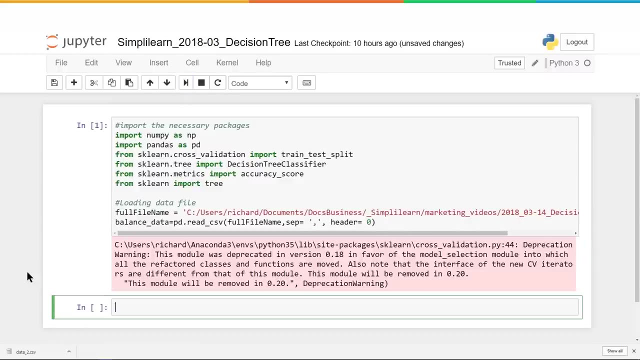 And then if I'm going to give it a name- full file name- I'm going to go ahead and change it here To full file name. So let's go ahead and run it now and see what happens And we get a warning. 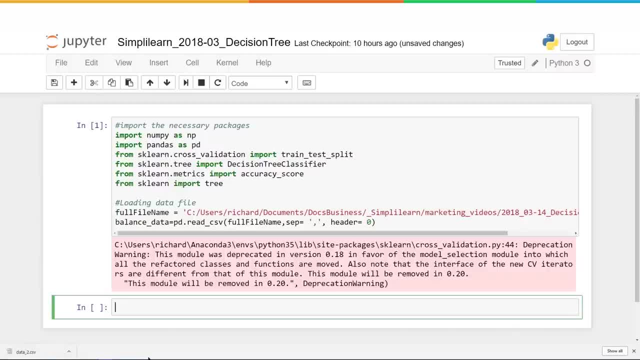 When you're coding, understanding these different warnings and these different errors that come up is probably the hardest lesson to learn. So let's just go ahead and take a look at this and use this as an opportunity to understand what's going on here. If you read the warning, 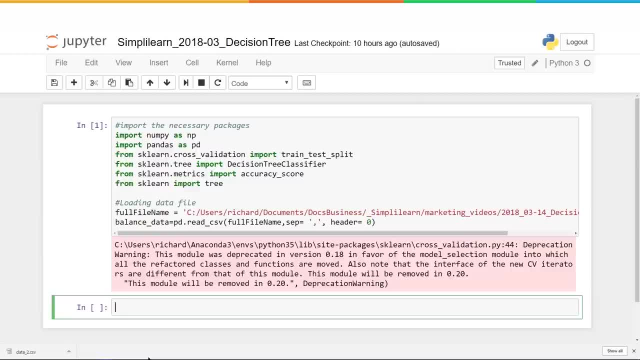 it says the cross-validation is depreciated. So it's a warning on it's being removed And it's going to be moved in favor of the model selection. So if we go up here, we have sklearncrossvalidation and if you research this and go to the sklearn site, 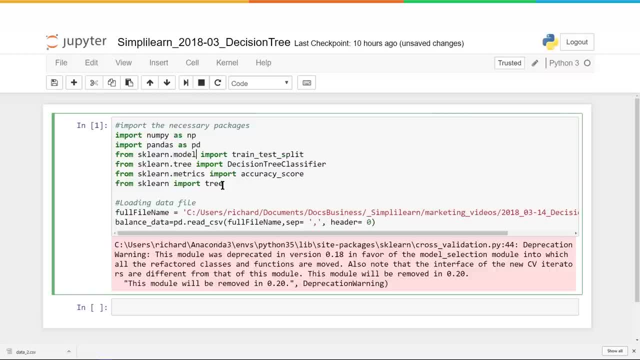 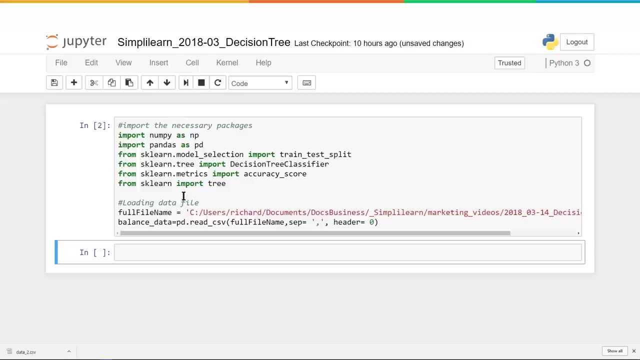 you'll find out that you can actually just swap it right in there with model selection, And so when I come in here and I run it again, that removes a warning. What they've done is they've had two different developers develop it in two different branches. 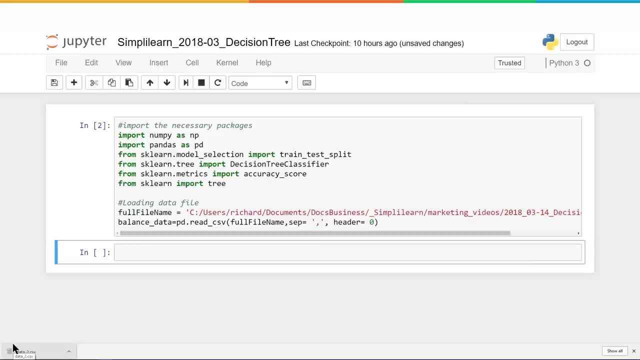 And then they decided to keep one of those and eventually get rid of the other one. That's all that is, And very easy and quick to fix. Before we go any further, I went ahead and opened up the data from this file. Remember the data file we just loaded on here? 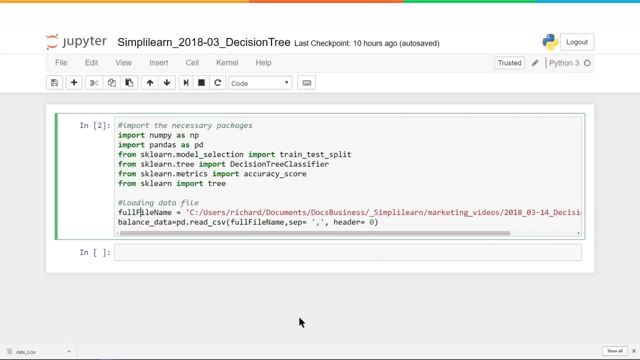 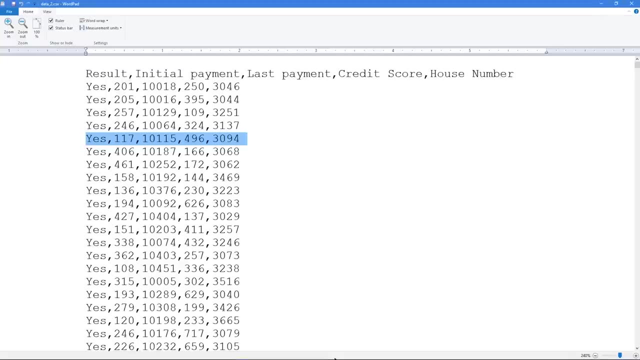 The data underscore two dot csv. Let's talk a little bit more about that and see what that looks like both as a text file and in a spreadsheet. This is what it looks like as a basic text file. You can see at the top they've created a header. 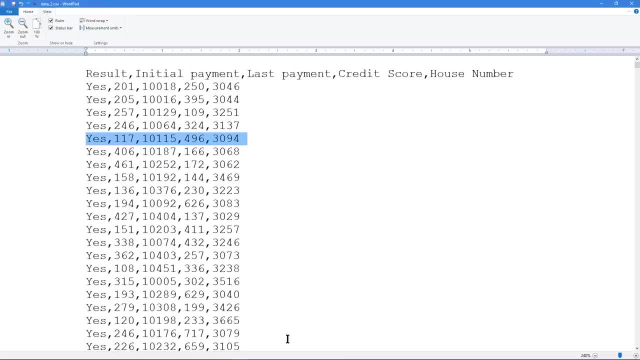 and it's got one, two, three, four, five columns And each column has data in it. And let me flip this over, because we're also going to look at this in an actual spreadsheet so you can see what that looks like. 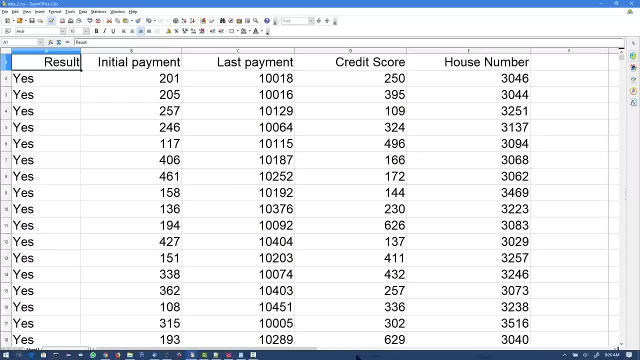 And here I've opened it up in the open office, calc, which is pretty much the same as Excel, And zoomed in and you can see we've got our columns and our rows of data A little easier to read. in here We have a result. yes, yes, no. 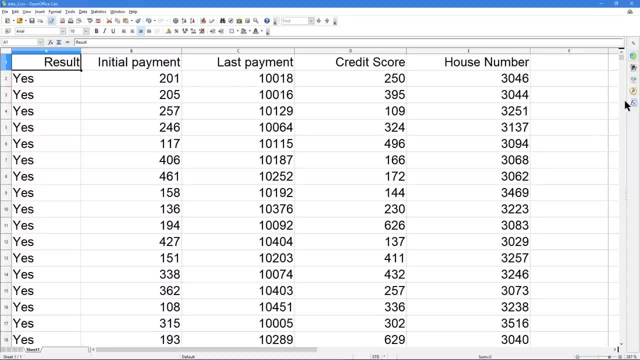 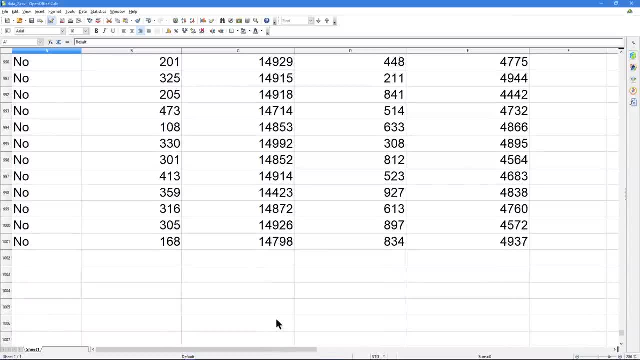 Initial payment. last payment: credit score: house number. If we scroll way down, we'll see that this occupies a thousand and one lines of code or lines of data, With the first one being a column and then one thousand lines of data. 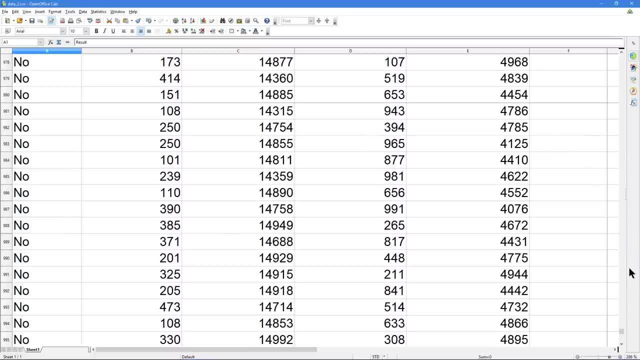 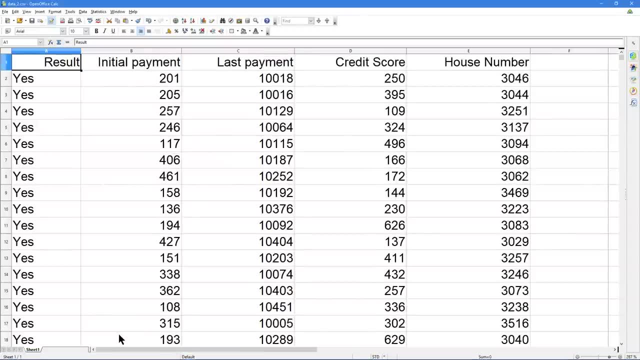 Now, as a programmer, if you're looking at a small amount of data, I usually start by pulling it up in different sources so I can see what I'm working with. But in larger data you won't have that option, It'll just be too large. 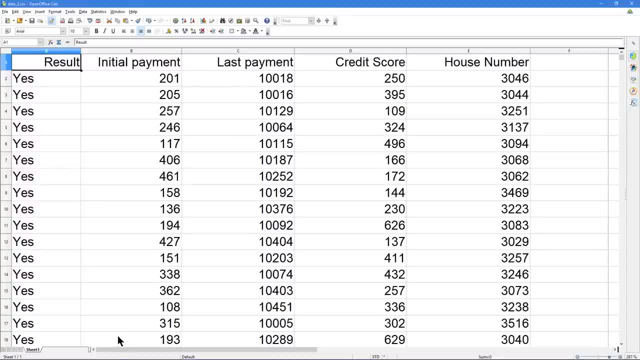 So you need to either bring in a small amount that you can look at it like we're doing right now, or we can start looking at it through the Python code. So let's go ahead and move on and take the next couple steps to explore the data using Python. 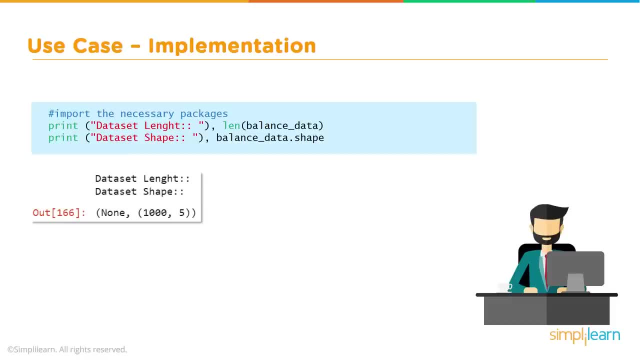 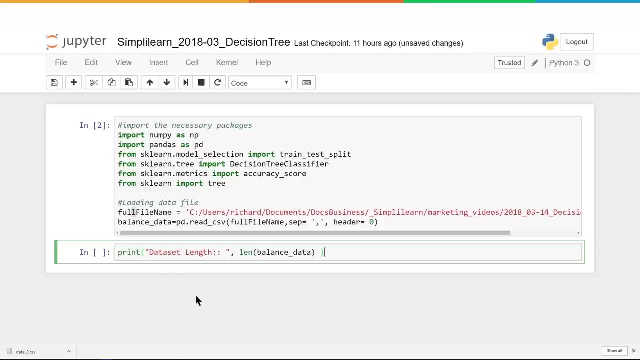 Let's go ahead and see what it looks like in Python to print the length and the shape of the data. So let's start by printing the length of the database. We can use a simple lin function from Python And when I run this you'll see that it's a thousand long. 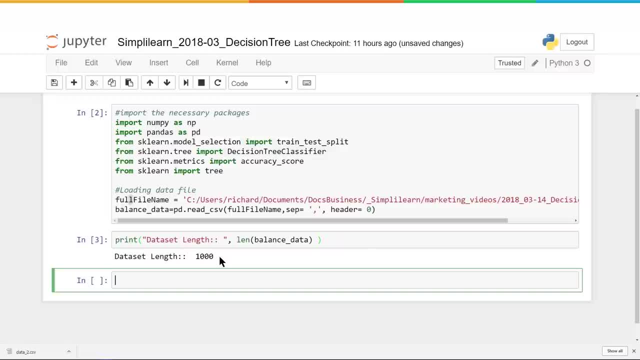 And that's what we expected. There's a thousand lines of data in there. if you subtract the column head- This is one of the nice things when we did the balance data from the Panda Read CSV- you'll see that the header is row zero, so it automatically removes a row. 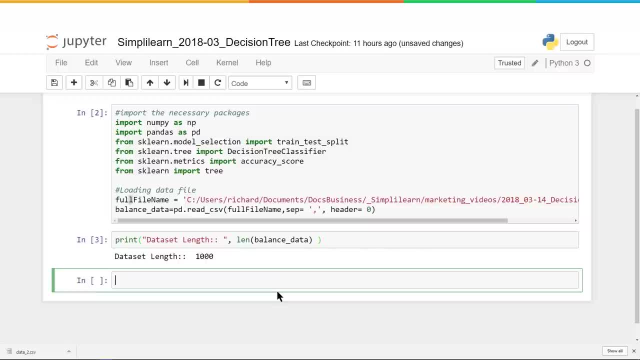 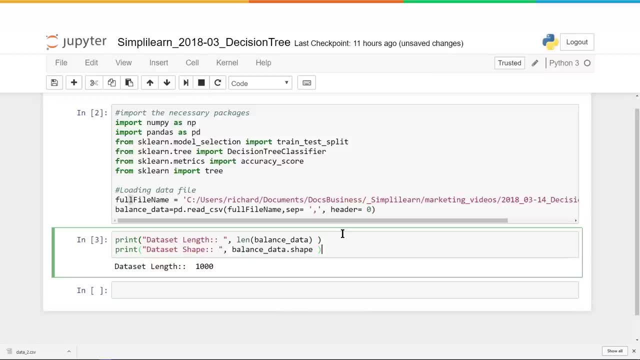 and then shows the data separate. It does a good job sorting that data out for us, And then we can use a different function. and let's take a look at that. And again, we're going to utilize the tools in Panda And since the balance underscore, 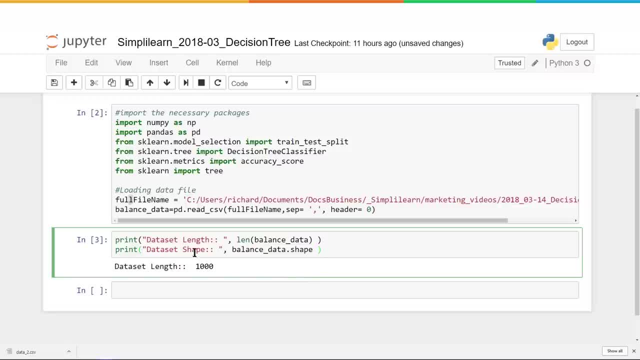 data was loaded as a Panda data frame. we can do a shape on it, And let's go ahead and run the shape and see what that looks like. What's nice about this shape is not only does it give me the length of the data, we have a thousand lines. 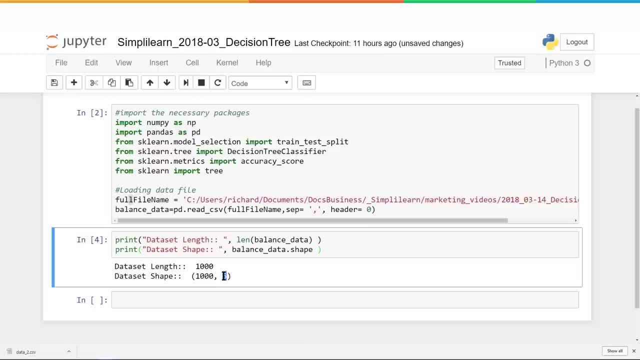 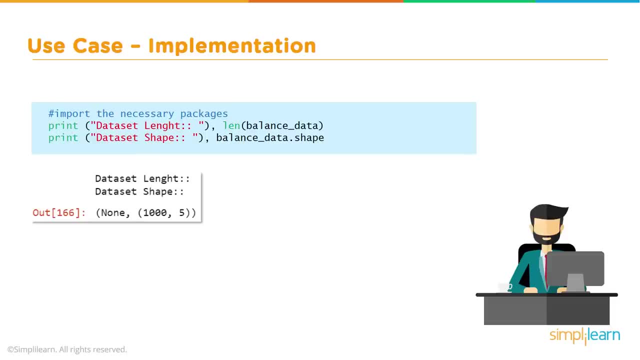 it also tells me there's five columns. So when we were looking at the data, we had five columns of data. And then let's take one more step to explore the data using Python. And now that we've taken a look at the length and the shape, 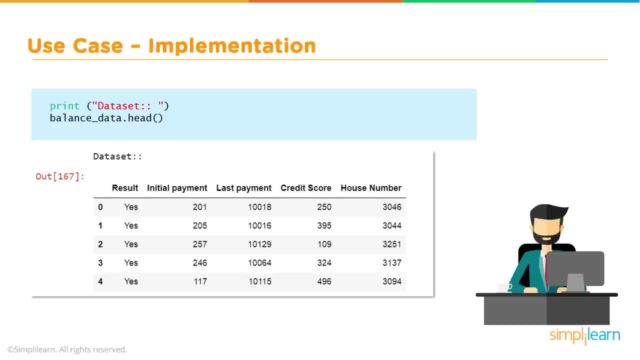 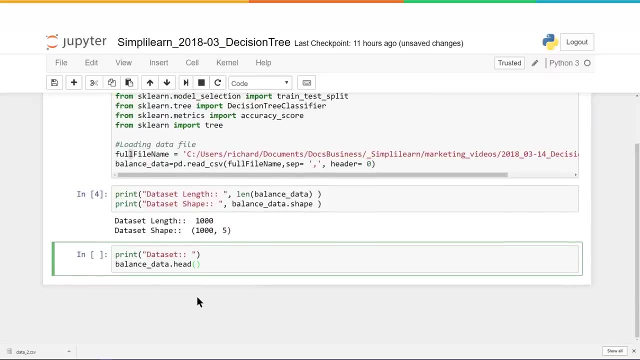 let's go ahead and use the Pandas module for head- Another beautiful thing in the data set that we can utilize. So let's put that on our sheet here and we have print data set and balance data dot head, And this is a Pandas. 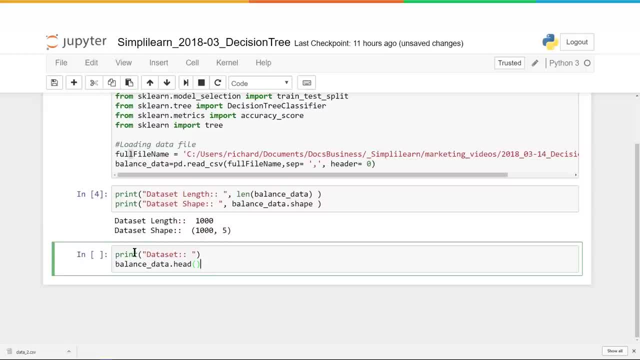 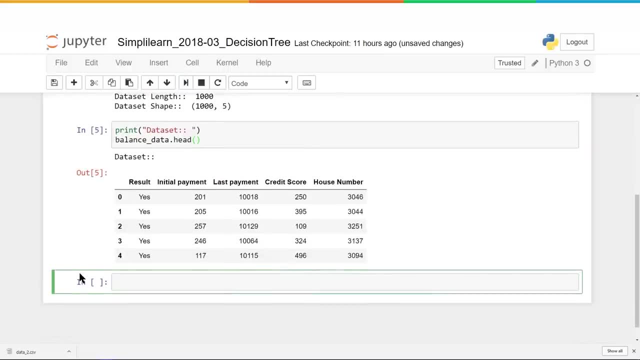 print statement of its own, So it has its own print feature in there. And then we went ahead and gave a label for our print job here of data set, Just a simple print statement. And when we run that and let's just take a closer look at that, 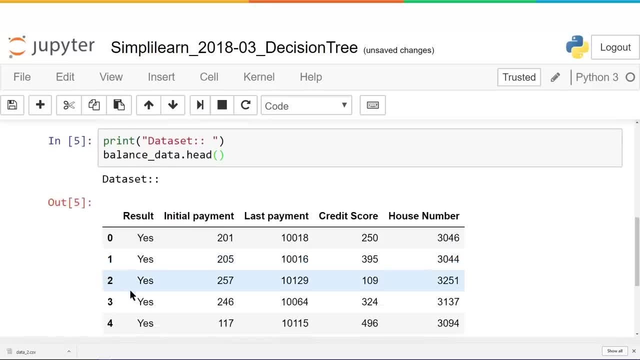 Let me zoom in here. There we go. Pandas does such a wonderful job of making this a very clean, readable data set, So you can look at the data. you can look at the column headers. you can have it when you put it as the head. 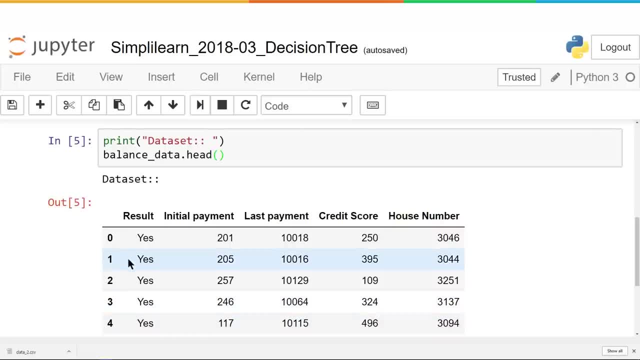 it prints the first five lines of the data And we always start with zero. So we have five lines. we have 0, 1,, 2,, 3, 4 instead of 1,, 2,, 3, 4, 5.. 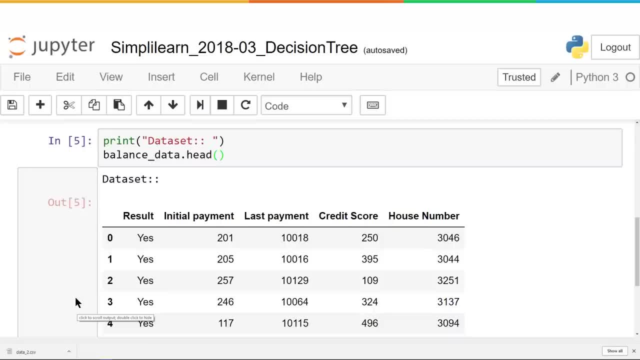 That's a standard scripting and programming set. is you want to start with the zero position? And that is what the data head does. It pulls the first five rows of data, puts it in a nice format that you can look at and view. Very powerful tool. 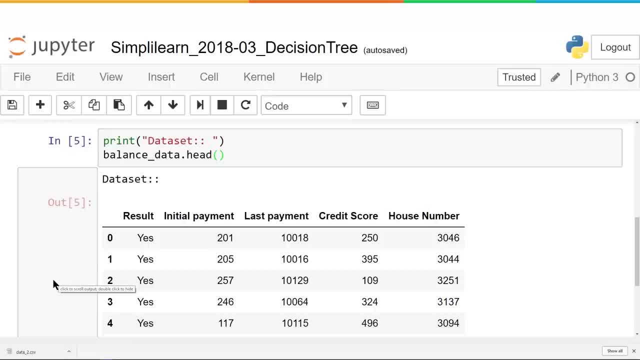 to view the data. So instead of having to flip and open up an Excel spreadsheet or open OfficeCal, or trying to look at a Word doc where it's all scrunched together and hard to read, you can now get a nice open view of what you're working with. We're 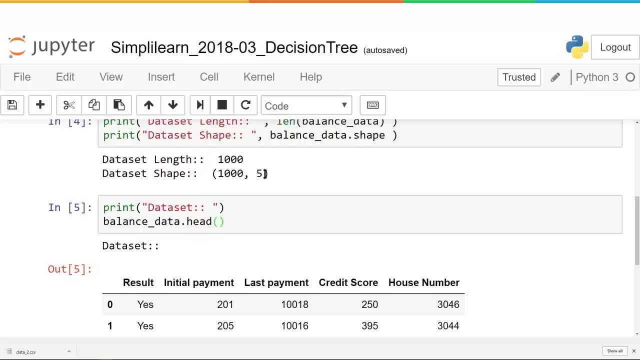 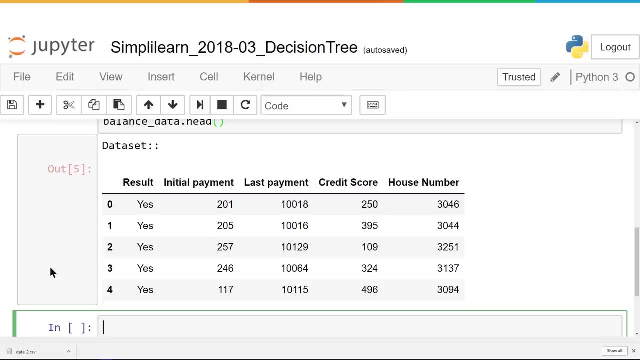 working with a shape of a thousand long, five wide, so we have five columns And we do the full data head. you can actually see what this data looks like: The initial payment, last payment, credit scores, house number. So let's. 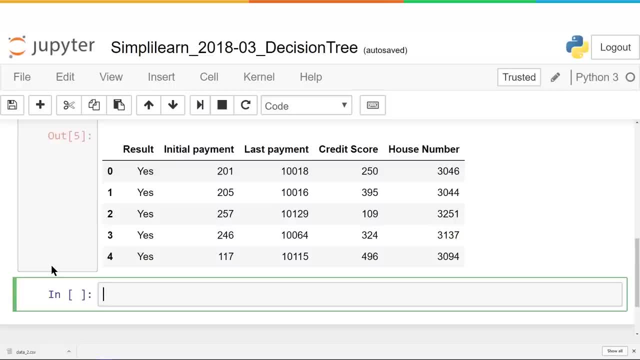 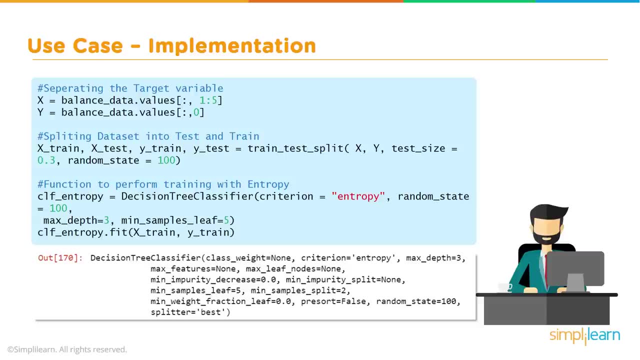 take this: now that we've explored the data, and let's start digging into the decision tree. So in our next step, we're going to train and build our data tree, And to do that, we need to first separate the data out. We're going to 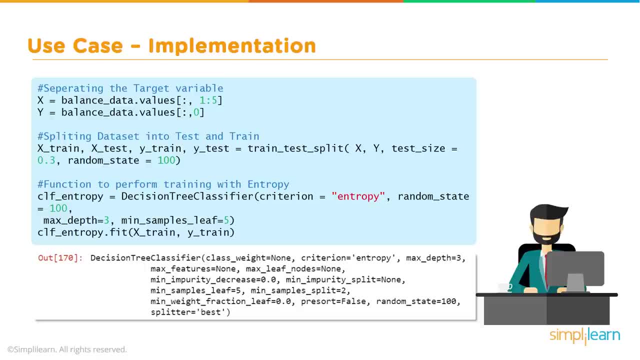 separate it into two groups so that we have something to actually train the data with, and then we have some data on the side to test it, to see how good our model is. Remember, with any of the machine learning, you always want to have some kind of test set. 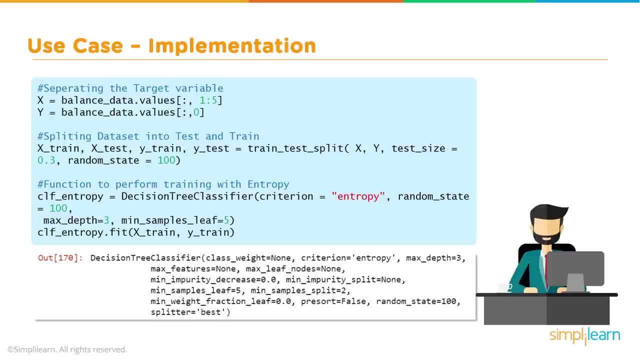 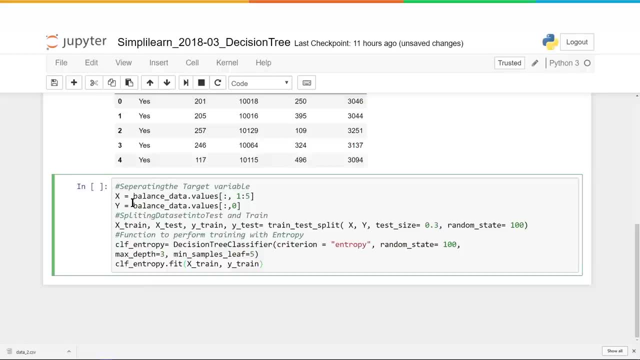 to weigh it against. so you know how good your model is when you distribute it. Let's go ahead and break this code down and look at it in pieces. So first we have our x and y. Where do x and y come from? Well, x is going to be. 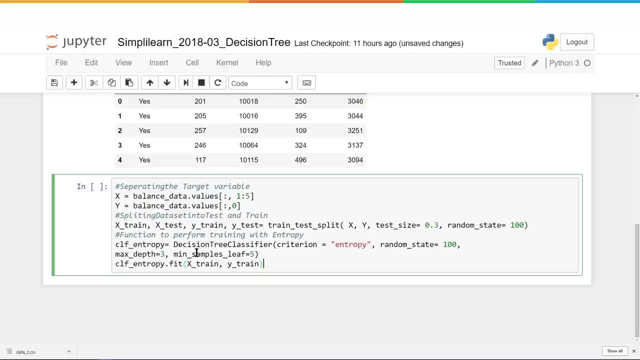 our data and y is going to be the answer or the target. You can look at it as source and target. In this case, we're using x and y to denote the data in and the data that we're actually trying to guess what the answer. 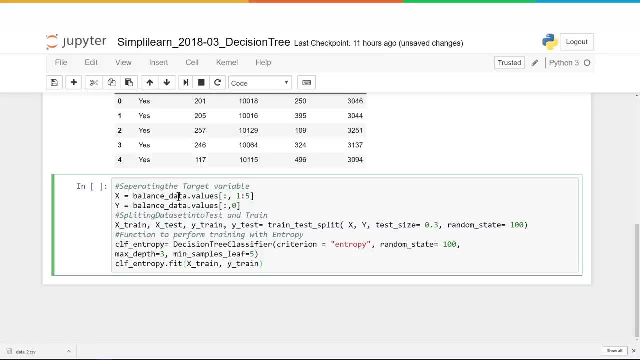 is going to be, And so to separate it we can simply put in: x equals the balance of the data, dot values, and the first brackets means that we're going to select all the lines in the database. So it's all the data. And the second one says we're only going to look at. 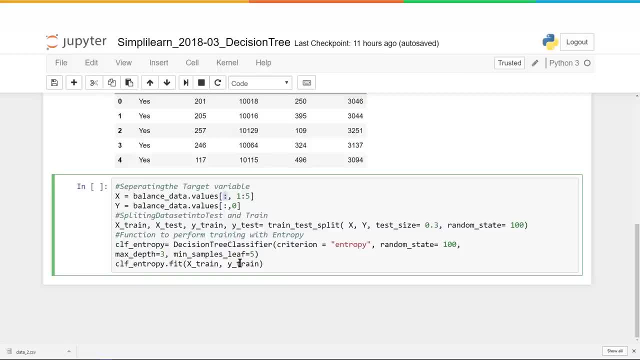 columns 1 through 5.. Remember, we always start with 0?. 0 is a yes or no and that's whether the loan went default or not. So we want to start with 1.. If we go back up here, that's the initial. 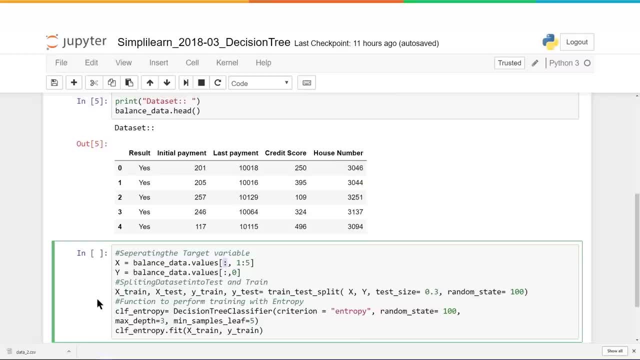 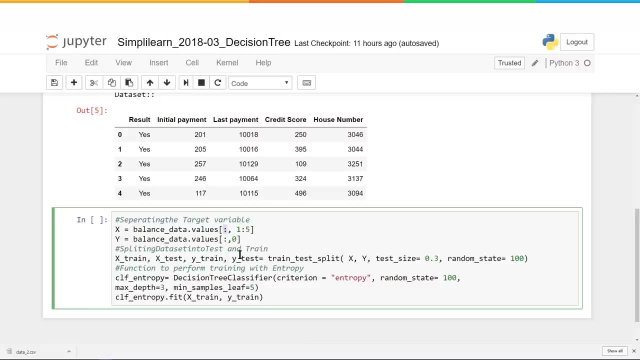 payment, and it goes all the way through the house number. Well, if we want to look at 1 through 5, we can do the same thing for y, which is the answer, and we're going to set that just equal to the 0 row. 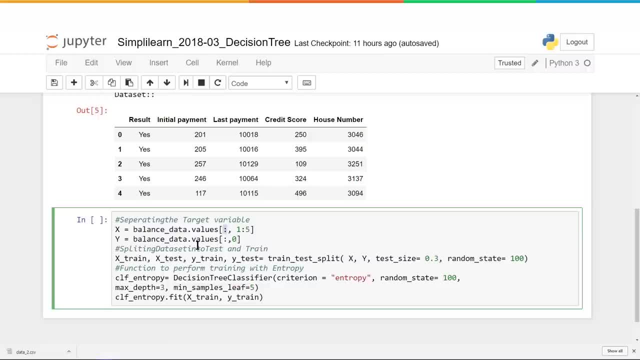 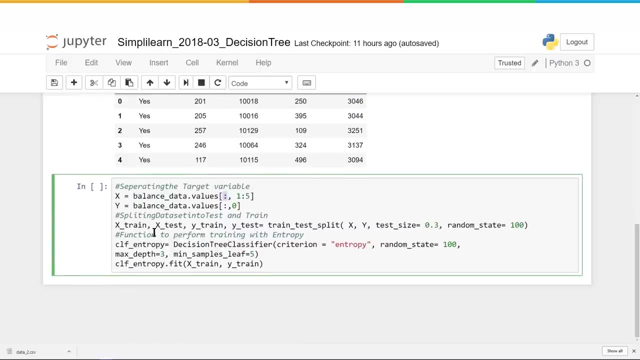 So it's just the 0 row and then it's all rows going in there. So now we've divided this into two different data sets, One of them with the data going in and one with the answers. Next we need to split the data. 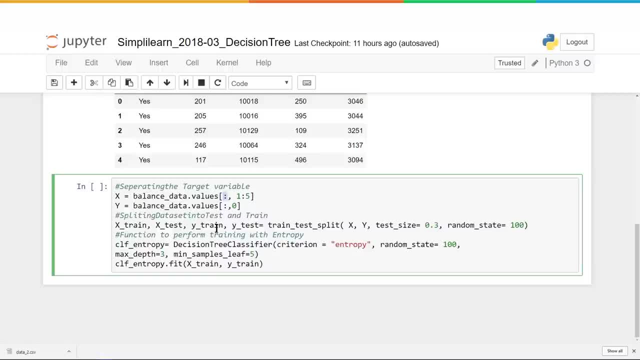 And here you'll see that we have it split into four different parts. The first one is your x training, your x test. your y train, your y test. Simply put, we have x going in where we're going to train it and we have to know the answer. 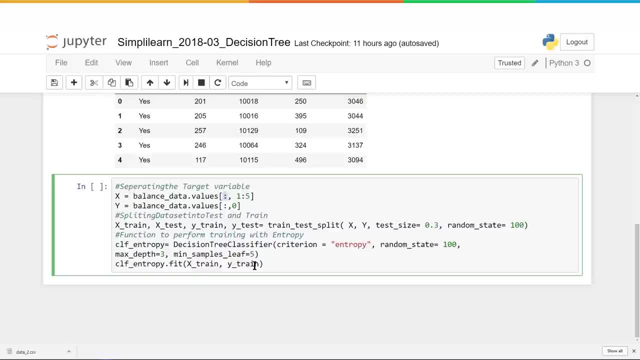 to train it with. And then we have x test, where we're going to test that data, And we have to know in the end what the y was supposed to be. And that's where this train test split comes in that we loaded earlier in the modules. 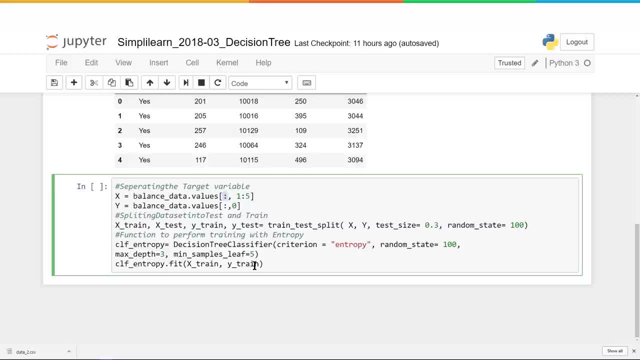 This does it all for us And you can see they set the test size equal to 0.3, so that's roughly 30% will be used in the test, And then we use a random state. so it's completely random which. 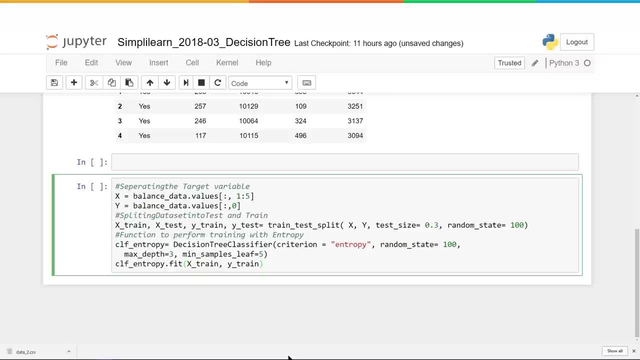 rows it takes out of there And then finally we get to actually build our decision tree And they've called it here clf underscore entropy. That's the actual decision tree or decision tree classifier, And in here they've added a couple variables which we'll explore. 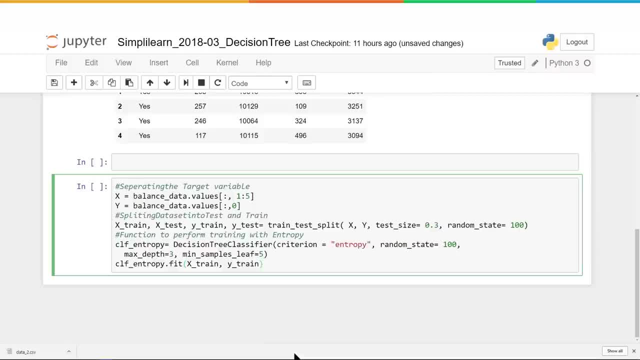 in just a minute. And then, finally, we need to fit the data to that. So we take our clf entropy that we created and we fit the x train and since we know the answers for x train are the y train, we go ahead and put those in And let's go ahead. 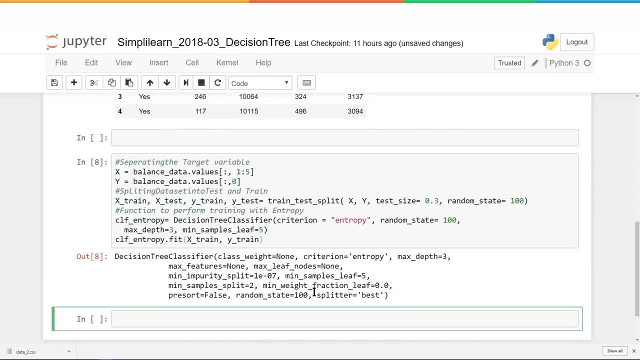 and run this, And what most of these sklearn modules do is when you set up the variable- in this case we set the clf entropy equal decision tree classifier- it automatically prints out what's in that decision tree. There's a lot of variables you can play with in here. 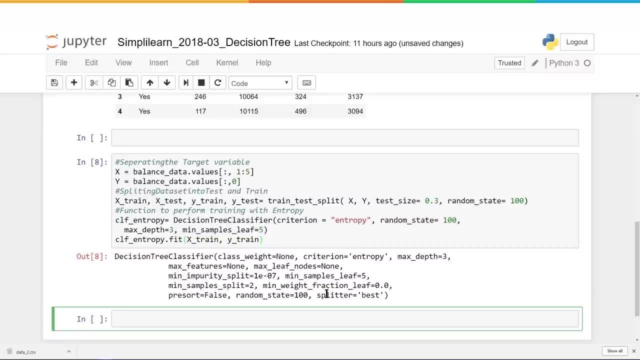 And it's quite beyond the scope of this tutorial to go through all of these and how they work. But we're working on entropy. that's one of the options We've added that it's completely a random state of 100, so 100%. 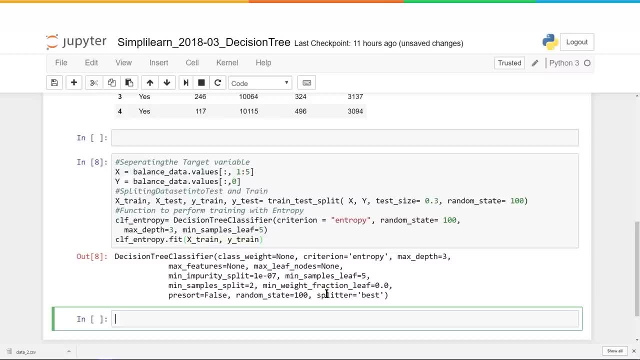 And we have a max depth of 3. Now, the max depth, if you remember above when we were doing the different graphs of animals, means it's only going to go down 3 layers before it stops, And then we have minimal samples of leaves as 5.. 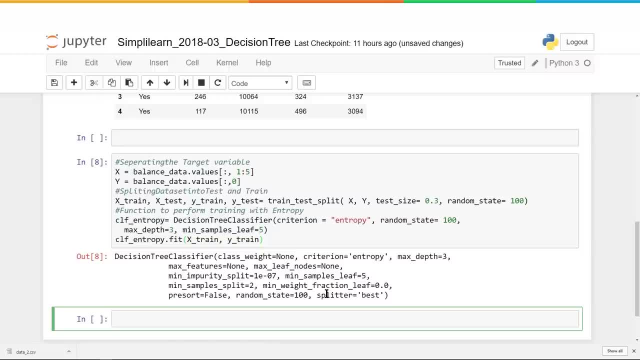 So it's going to have at least 5 leaves at the end. So it'll have at least 3 splits. it'll have no more than 3 layers and at least 5 end leaves, with the final result at the bottom, Now that we've created. 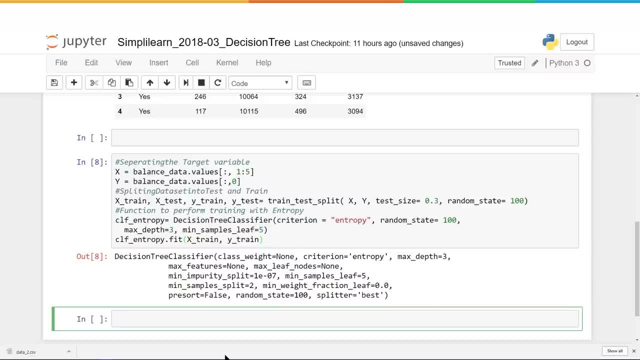 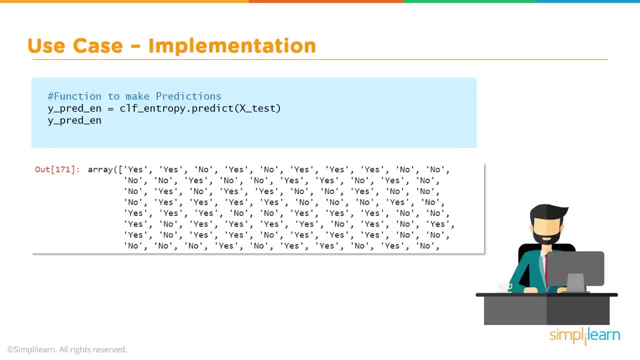 our decision tree classifier not only created it, but trained it. let's go ahead and apply it and see what that looks like. So let's go ahead and make a prediction and see what that looks like. We're going to paste our predict code in here. 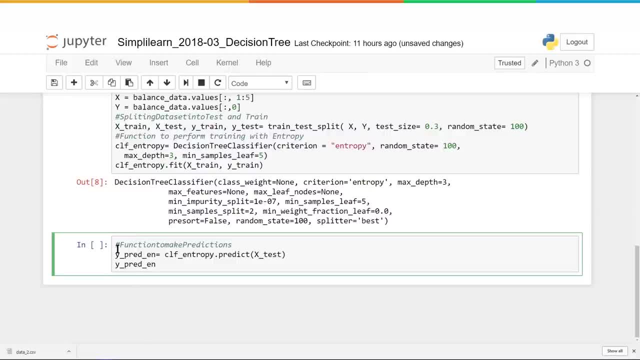 And before we run it, let's just take a quick look at what it's doing. here We have a variable ypredict that we're going to do And we're going to use our variable clfentropy that we created, And then you'll see. 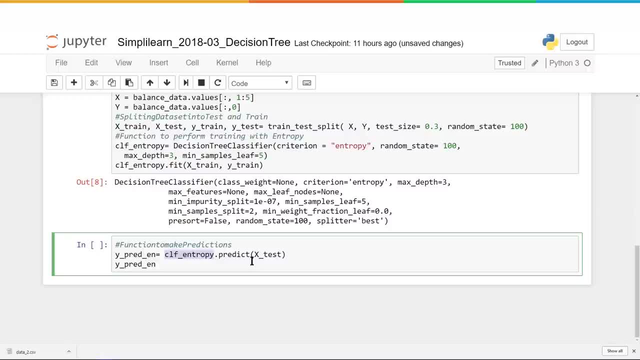 predict, And it's very common in the sklearn modules that their different tools have the predict when you're actually doing a prediction. In this case, we're going to put our xtestdata in here Now, if you delivered this for use- an actual commercial use- 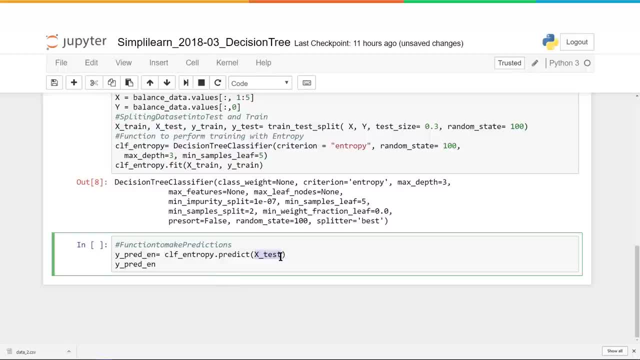 and distributed it. this would be the new loans you're putting in here. to guess whether the person's going to be pay them back or not, In this case we need to test out the data and just see how good our sample is, how good our tree does. 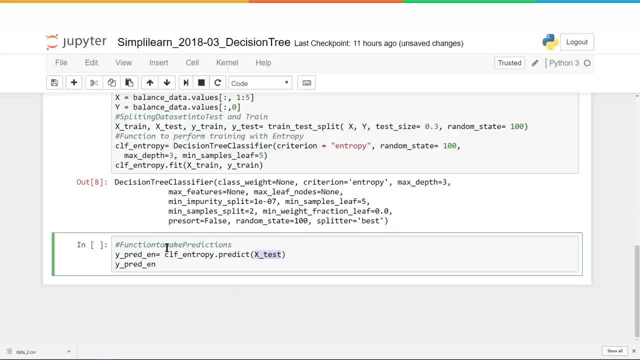 at predicting the loan payments. And finally, since Anaconda Jupyter Notebook works as a command line for Python, we can simply put the ypredicten to print it. I could just as easily have put the print and put brackets around ypredicten. 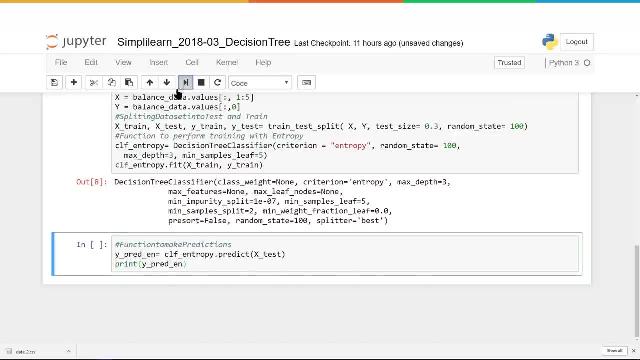 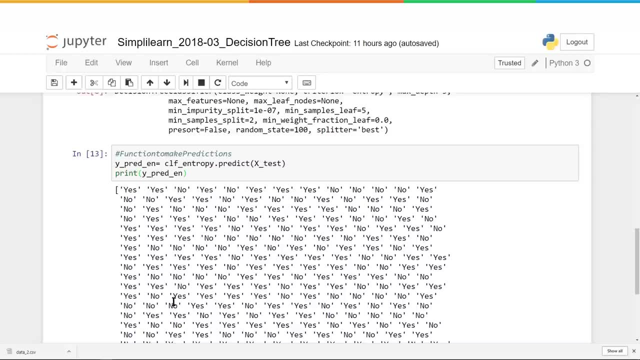 to print it out. We'll go ahead and do that. It doesn't matter which way you do it, And you'll see right here that it runs a prediction. This is roughly 300 in here. Remember it's 30% of 1000, so you should have. 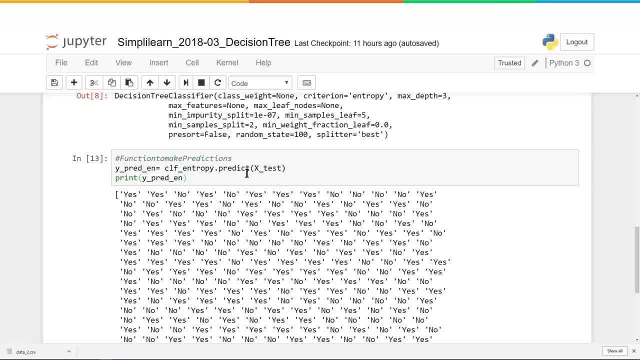 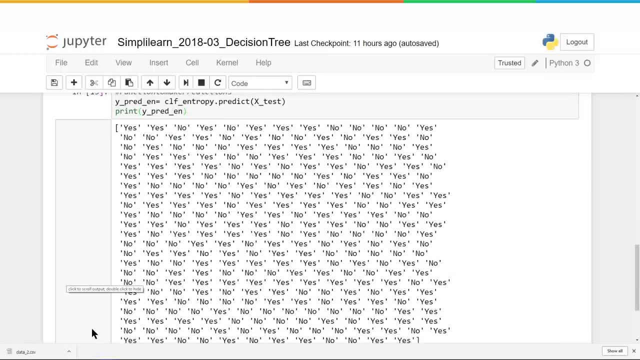 about 300 answers in here, And this tells you which each one of those lines of our test went in there, and this is what our ypredict came out. So let's move on to the next step. We're going to take this data and try to figure out. 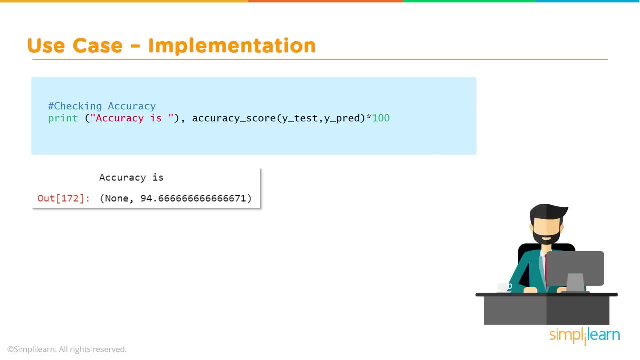 just how good a model we have. So here we go. Since sklearn does all the heavy lifting for you and all the math, we have a simple line of code to let us know what the accuracy is, And let's go ahead and go through that and see what that. 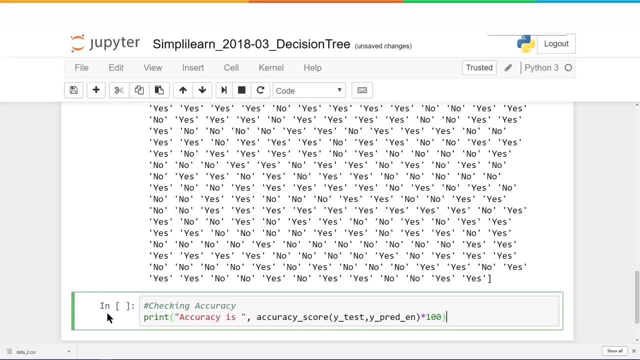 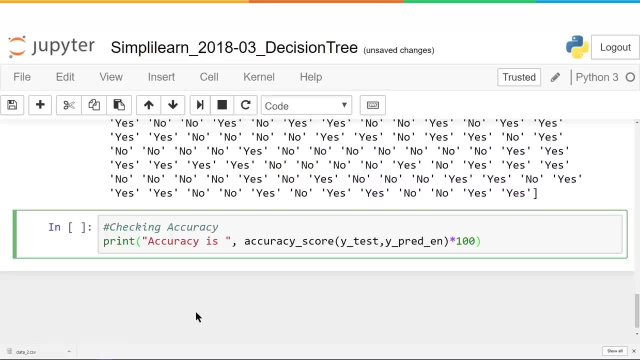 means and what that looks like. Let's go ahead and paste this in And let me zoom in a little bit. There we go, See we have a nice full picture And we'll see. here we're just going to do a print. accuracy is. 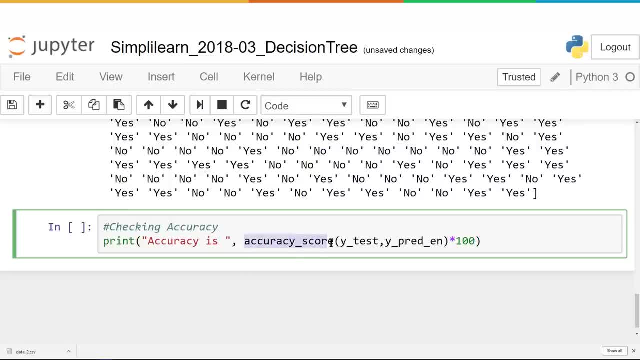 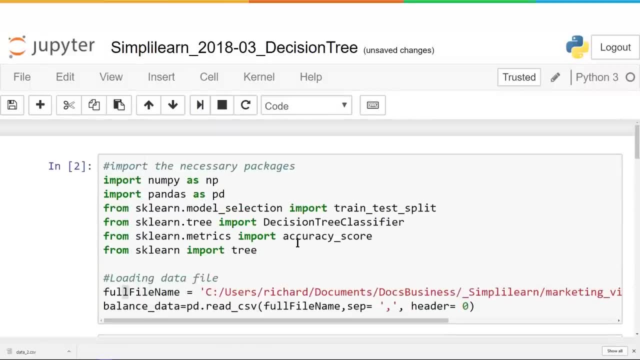 And then we do the accuracy score And this was something we imported earlier, if you remember, at the very beginning. Let me just scroll up there real quick so you can see where that's coming from. That's coming from here, down here, from sklearnmetrics import. 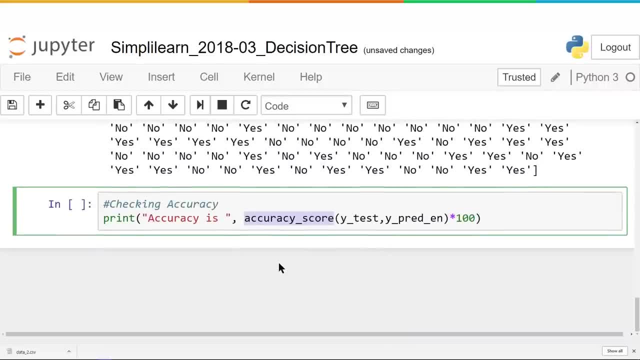 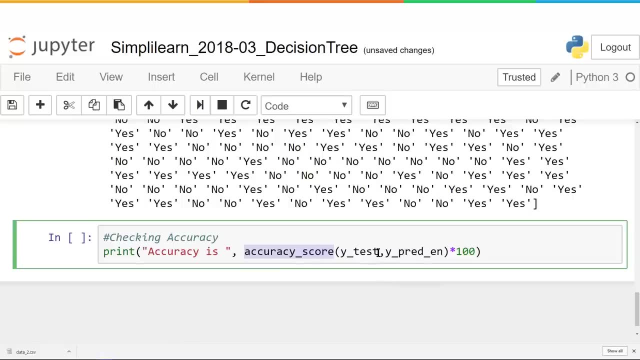 accuracy score, And you could probably run a script, make your own script, to do this very easily. How accurate is it? How many out of 300 do we get right? And so we put in our ytest? That's the one we. 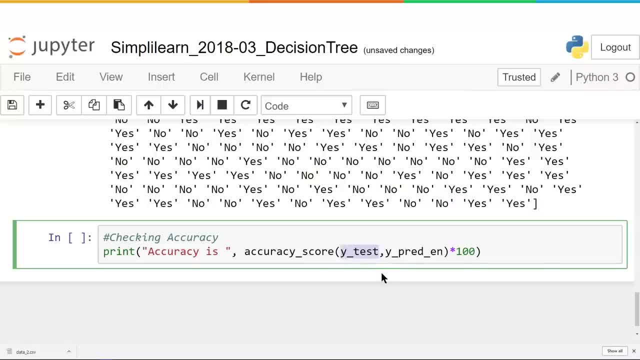 ran the predict on And then we put in our ypredicten: That's the answers we got And we're just going to multiply that by 100. Because this is just going to give us an answer as a decimal And we want to see it as a percentage. 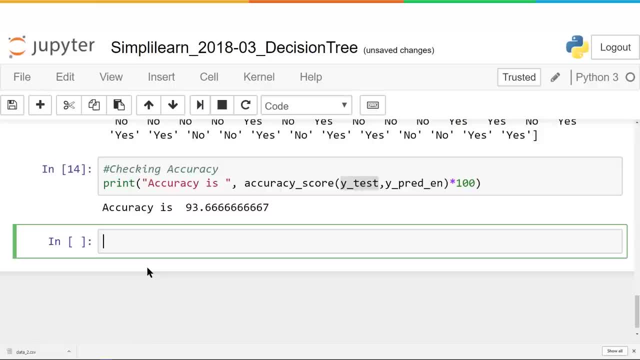 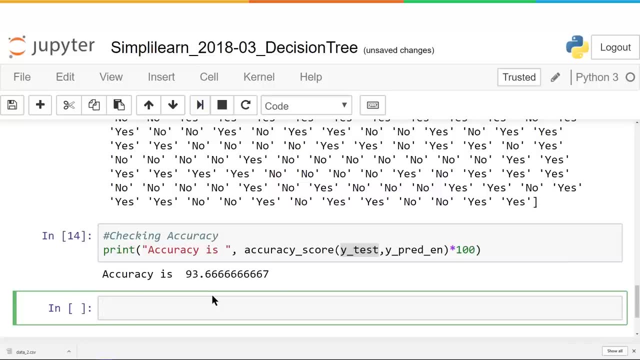 And let's run that and see what it looks like. And if you see, here we got an accuracy of 93.66667.. So when we look at the number of loans and we look at how good our model fit, we can tell people it has about a 93.6. 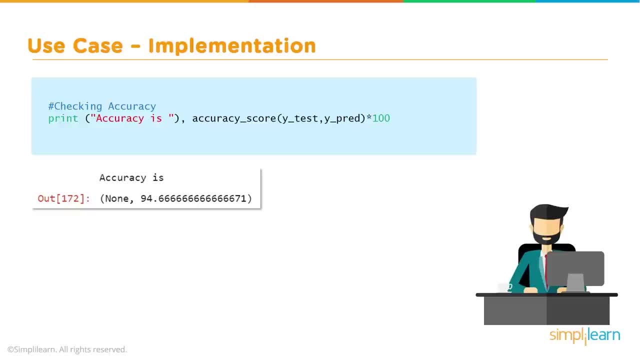 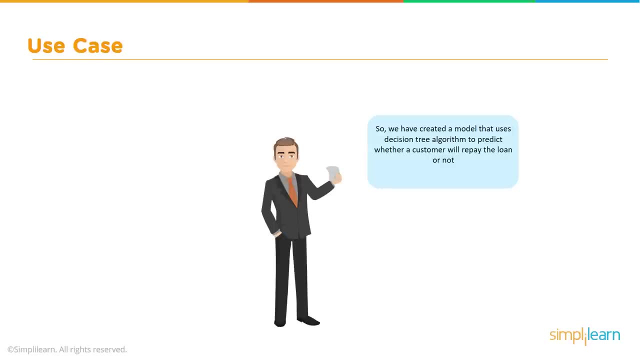 fitting to it. So just a quick recap on that. We now have accuracy set up on here, And so we have created a model that uses the decision tree algorithm to predict whether a customer will repay the loan or not. The accuracy of the model is about 94.6%. 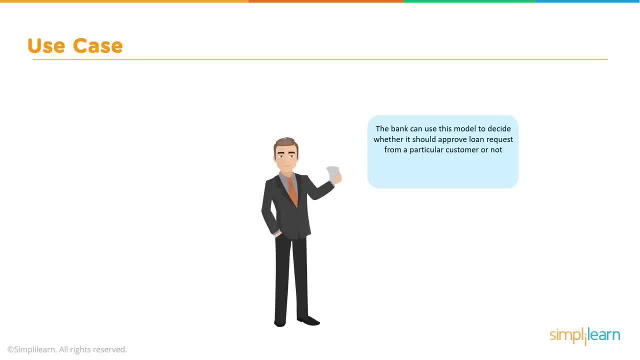 The bank can now use this model to decide whether it should approve the loan request from a particular customer or not, And so this information is really powerful. We may not be able to, as individuals, understand all these numbers, because they have thousands of numbers that come in, But you can see that this is a smart 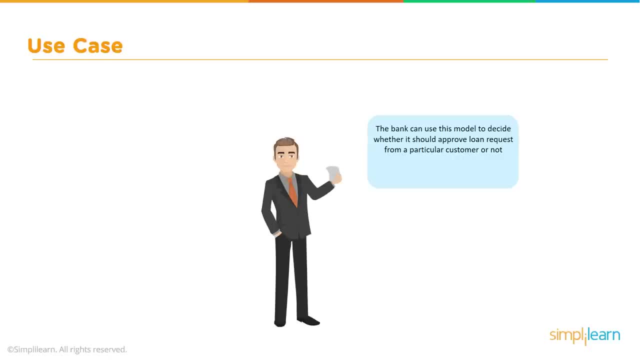 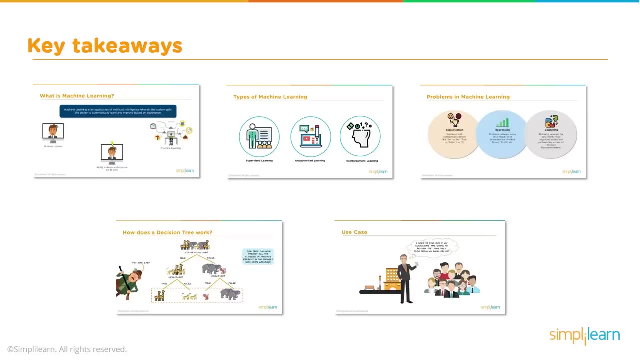 decision for the bank to use a tool like this to help them to predict how good their profit is going to be off of the loan balances and how many are going to default or not. So we've had a lot of fun learning about decision trees, So let's take a look at the key takeaways. 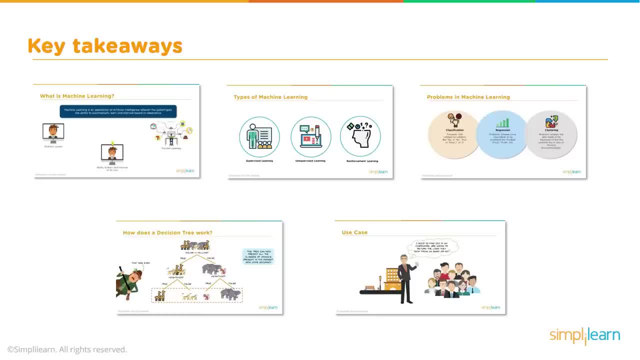 that we've covered today. What is machine learning? We covered up some different aspects of machine learning and what that is utilized in your everyday life and what you can use it for: For predicting, for describing, for guessing what the next outcome is, for.